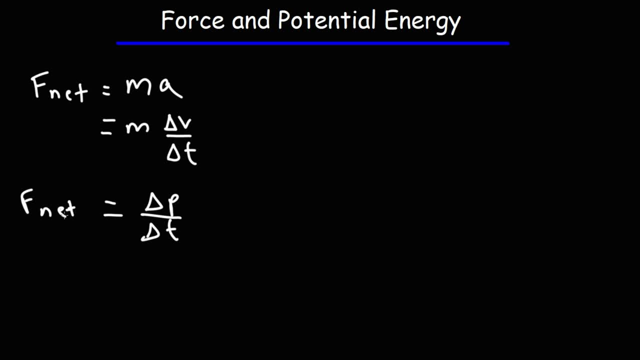 net force is equal to the mass times an object's acceleration, which is true. the net force of an object is also equal to the force acting on that object, multiplied by the object's acceleration, to the rate at which the momentum of that object is changing. In other words, 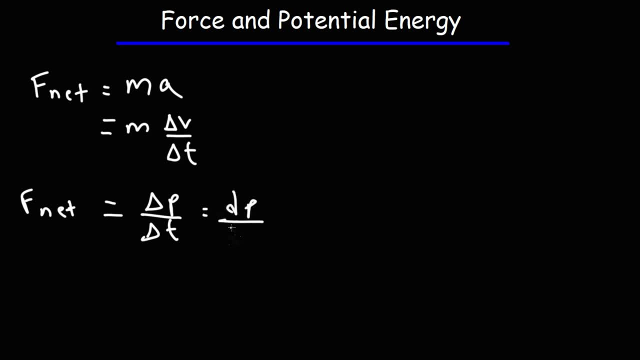 the net force is equal to the derivative of momentum function. So you can easily find the force function if you have the momentum function. But here's a key point that you want to keep in mind: It's with respect to time. So the net force acting on an object 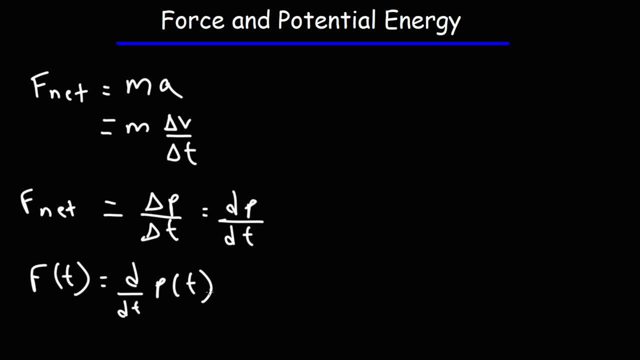 is the derivative of the momentum function with respect to time. Now we know that the work done by a conservative force is equal to the negative change in potential energy, And the work done by any force on an object is equal to the magnitude of that force. times. 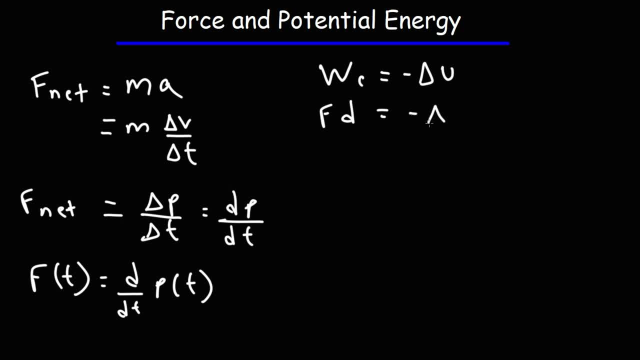 the displacement. So we could set that equal to the negative change in potential energy. If we divide both sides by the displacement, we get that force is equal to the negative change in potential energy divided by the object's displacement. Now let's say that force is in the x direction. 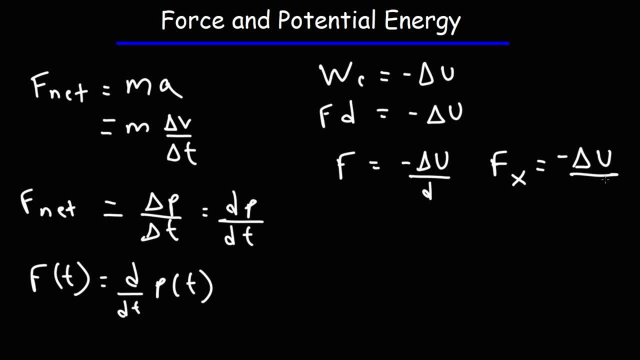 In this case, displacement will be the change in the object's position along the x-axis, So it's going to be delta x. So notice that the force function is basically the negative derivative of the potential function. But notice the difference between these two Net. 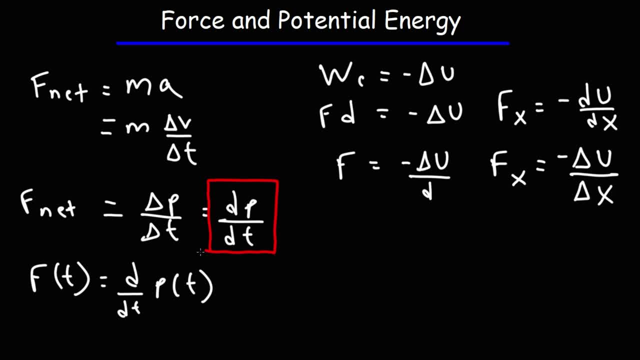 force is equal to the derivative of the momentum function with respect to time. Now the force is equal to the negative difference between these two. And the force acting on an object is equal to the negative change in potential energy derivative of the potential function, but not with respect to time, but with respect to position. so 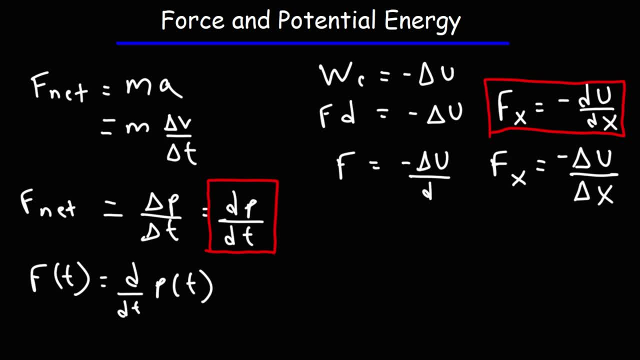 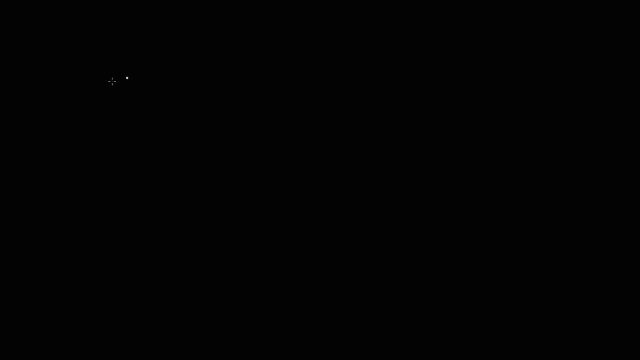 make sure you see that you understand that key difference there. so if you want to determine the force function, all you need to do is take the negative derivative of the potential function. now here's some other additional notes that you want to take down. whenever the force and 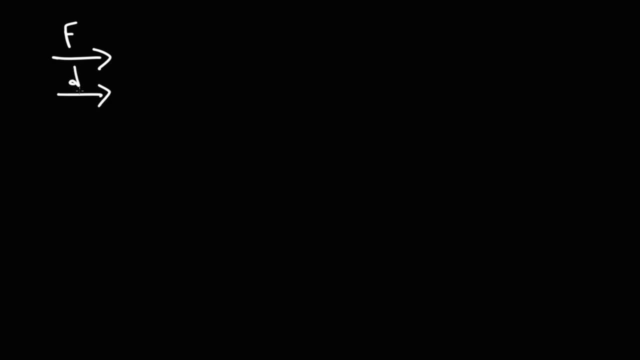 the displacement vectors when they're in the same direction, and this is within what we're talking about a conservative force here. when they're in the same direction, the work done by this force is positive. the kinetic energy of the object is going to increase because of the force and the displacement vectors are going to increase because of the force. 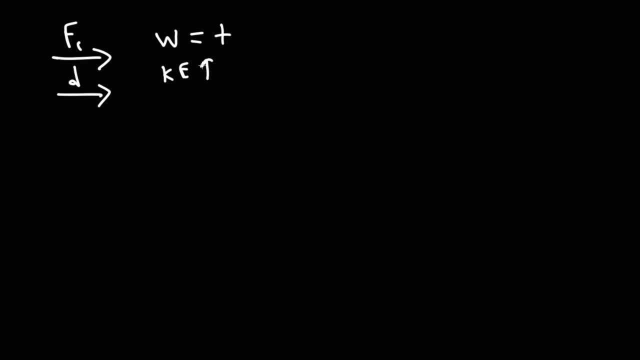 the force is accelerating the object, its velocity is increasing, and so it's kinetic energy is going to go up, but the potential energy is going to decrease. keep in mind: the network done on an object is equal to the change in the objects, kinetic energy and the work done. 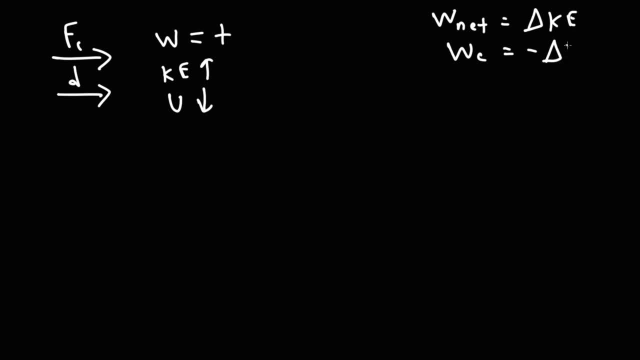 by a conservative force is equal to the negative change of the potential energy of that force, that object. so when kinetic energy goes up as the result of a conservative force acting on an object, the potential energy is gonna go down. what I want you to get from this is that when the force 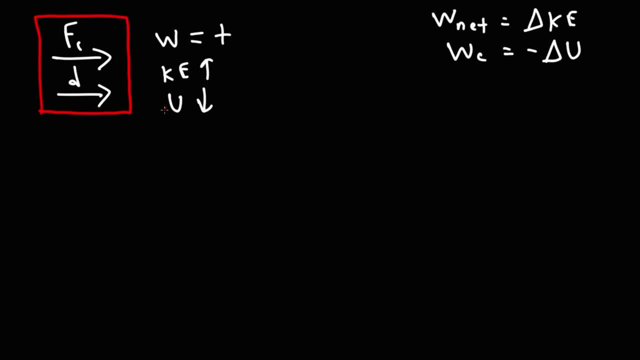 and the displacement vectors are parallel to each other, potential energy is gonna decrease. so if you're moving an object in the direction of the conservative force, the potential energy of that object is going to decrease. now the reverse is true when the object moves in the direction against the conservative force. 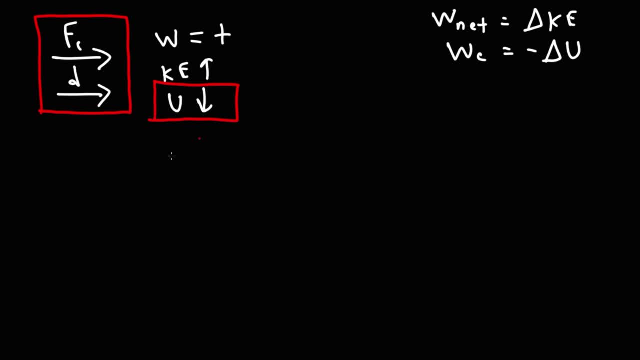 the potential energy of that object is going to go up. so let's say the conservative force is to the right but the object's displacement vector is to the left. the work done by this conservative force on the object is going to be negative because the force is. 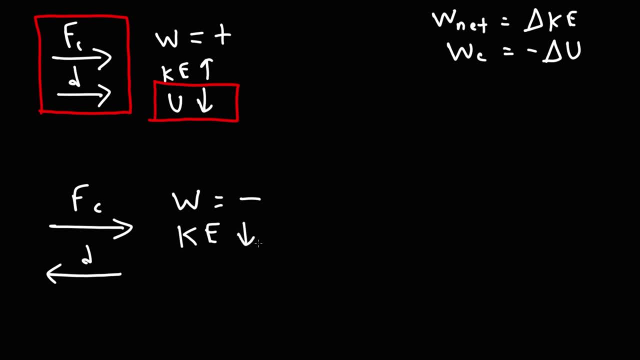 slowing it down, and so the kinetic energy is going to decrease. Now, because the conservative force is slowing it down, it's also increasing the object's potential energy, and we're going to consider a few examples of this truth. So make sure you understand that when the force, when the conservative force and the displacement 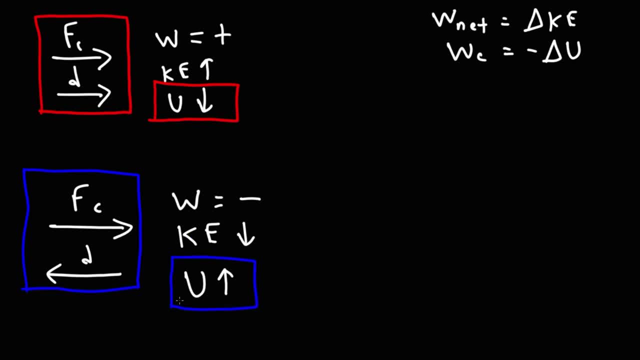 vectors are anti-parallel, potential energy goes up. When they're parallel, the potential energy goes down. So in the first scenario we're going to use gravity as our example. So let's say we have an object above ground level and we decide to let it go. 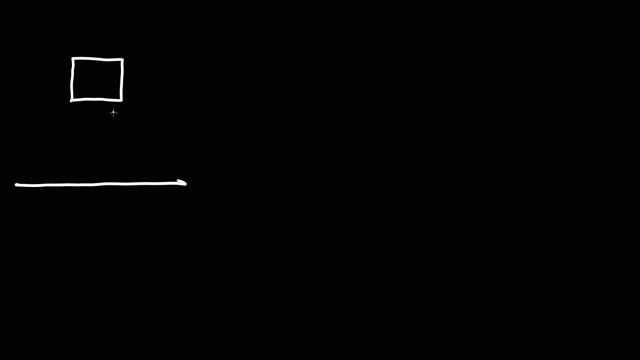 we release it from rest, well, the object's going to fall, so its displacement vector is going to be in the negative y direction. now the gravitational force is also in the negative y direction. I gotta put my phone on. silent is just making too much, too many noises. 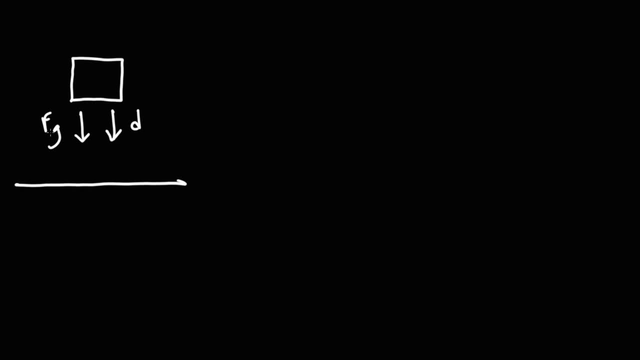 so notice in this example, force and the displacement vector. they're in the same direction. is the potential energy of the object going to increase or decrease? they're in the same direction. because the object is moving in the direction of the conservative force of gravity, the potential energy is going to decrease and we know this to be a case. 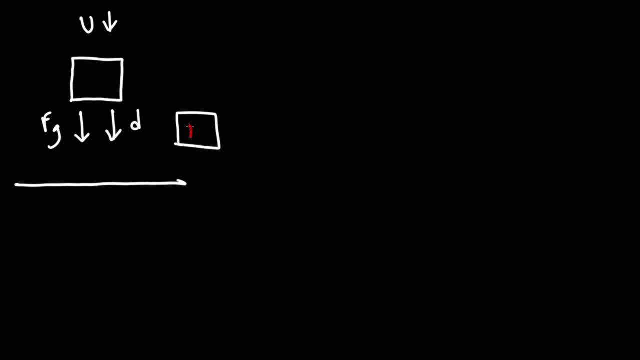 when the object is in position b here to position a, the potential energy at b is going to be lower than it is at a, because we know that potential energy is mgh. it's dependent on the height of the object. so a is at a greater height than position b and so object a is going to have 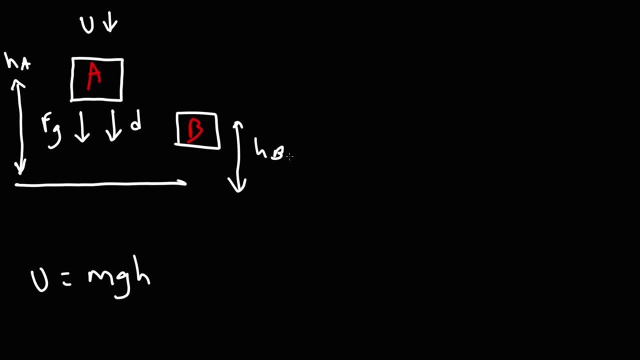 more potential energy, assuming the mass is the same. so when an object falls, its potential energy is decreasing, since b has less potential energy than a, but, as we could see, when the force and displacement values are in the same direction, the potential energy is going to decrease. if we're dealing with a conservative force, now, the reverse is true. let's say, if we were, 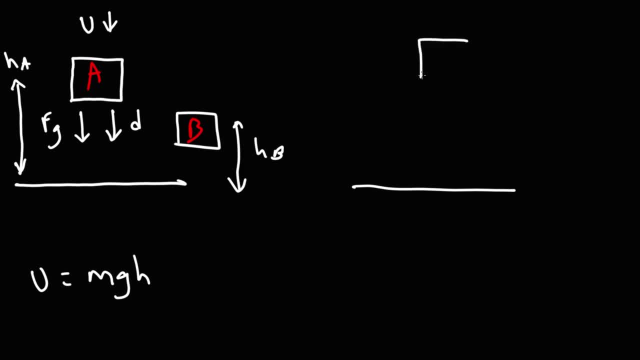 to move a to a higher position. as we move this block, gravity still wants to bring it down, but as we're lifting it up, its displacement vector is in the positive direction. so we're going to be using a positive y direction. so because these two vectors are opposite to each other, the potential energy is increasing. 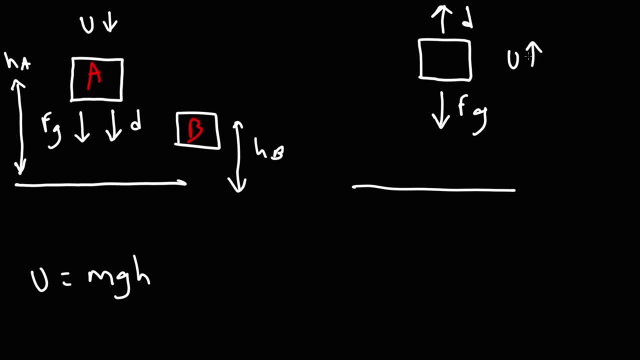 so, as we can see, whenever an object moves against a conservative force, its potential energy is increasing. now the next example we're going to consider is that of a spring. so let's say we have a spring that is pointing related to that virtual field in theечат, so we're choosing. that is also. 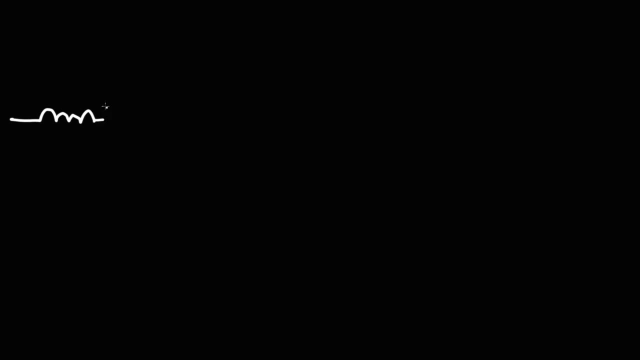 a variable that, missing, whether such a flat culture or not, have a spring that's been compressed from its natural length, And let's say the natural length is here. The spring wants to get back to this position, And so there's something called a restoring force that wants to bring it back to this position, But right now we are applying a 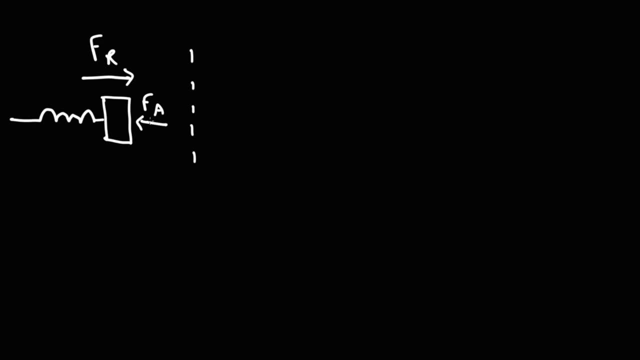 force to move it away from its natural position. So this spring it's still being compressed at the moment. So the displacement vector is going to be to the left. As we apply this force to the left, as we compress it against, the restoring force is the potential energy of the spring. 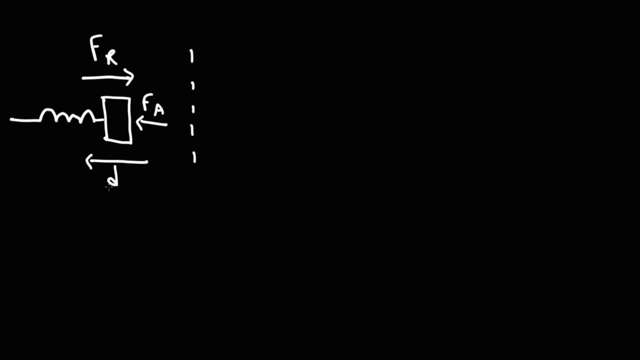 increasing or decreasing. What would you say? Now, the first thing we need to determine is if the displacement vector is parallel or anti-parallel to the conservative force. The conservative force in this example is not the applied force. That's something that we're doing. 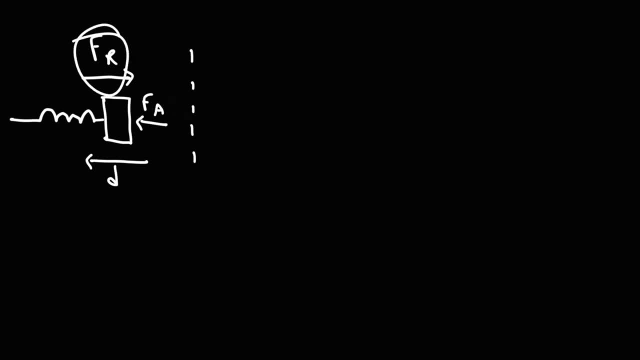 It is the restoring force, That is the conservative force that's acting in this spring, And notice that these two vectors are opposite in direction. Whenever you move the object against the conservative force, the potential energy will increase. Now we know the potential energy for. 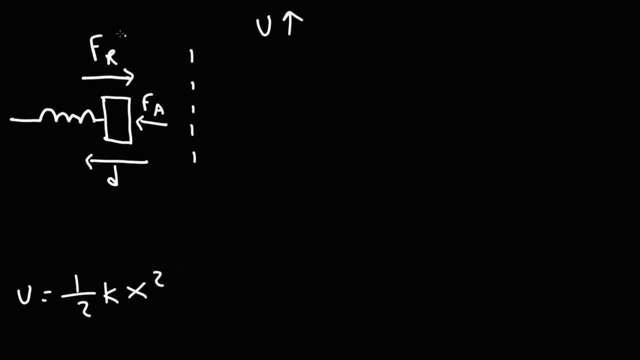 a spring is one half AX squared And X is the distance between the equilibrium point and the point where it's at rest and the current position, which is where it's currently compressed at. So as we move the object to the left, X is going to increase. And as X increases, 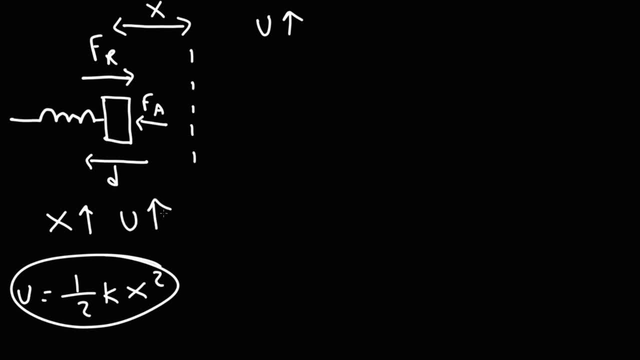 according to this equation, potential energy is going to go up. So in other words, we see another example that whenever we move an object against the conservative force, the potential energy is going to decrease. And we could look at this scenario in the other direction as well. 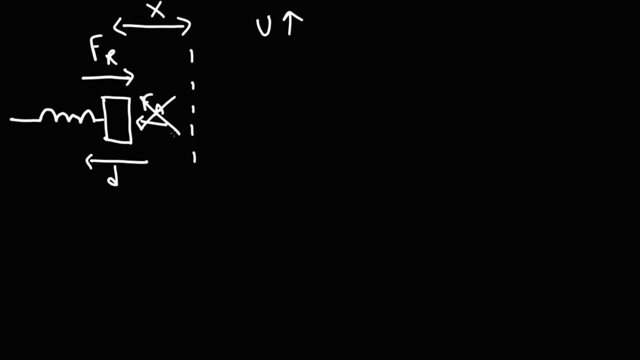 Let's say, if we get rid of the applied force, we're no longer trying to compress it, We are allowing the restoring force to do its thing. Once we remove the applied force and the restoring force takes over, the object will naturally move towards its equilibrium position. 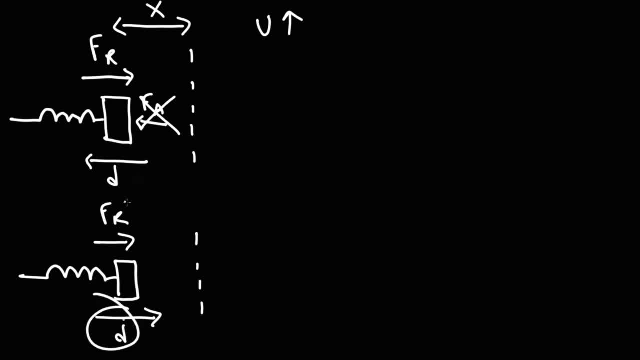 Now, in this case, because the object is moving in the direction of the conservative force, its potential energy will decrease. Now, because this conservative force, or the restoring force, is accelerating the object towards the equilibrium position, this force is doing positive work on the object. 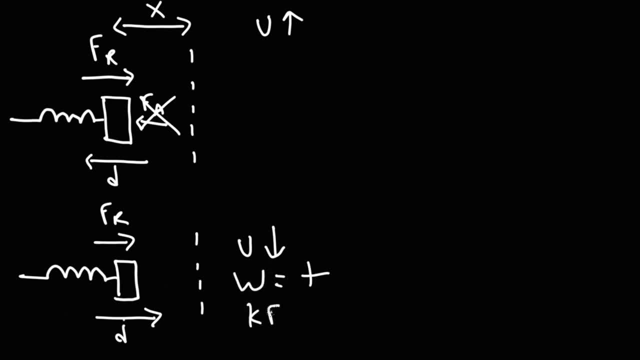 It's causing the object to speed up, and so its kinetic energy is going up. Now let's look at another example. Let's say we have a positively charged plate on one side and on this side a metal plate that is negatively charged. 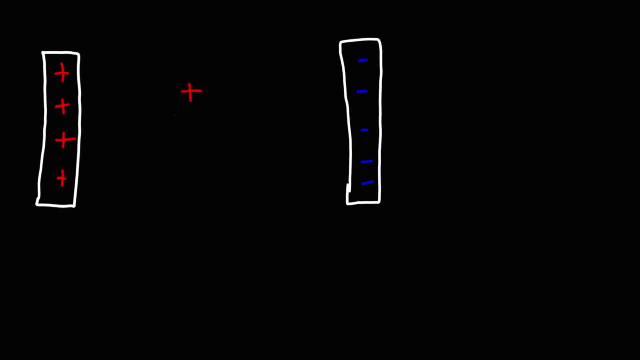 Now let's say we have a positive charge here. Now there is an electric field that points towards the positive plate and is directed to the negative plate. That electric field is equal to the force- the electric force acting on the charge- divided by the magnitude of that charge. 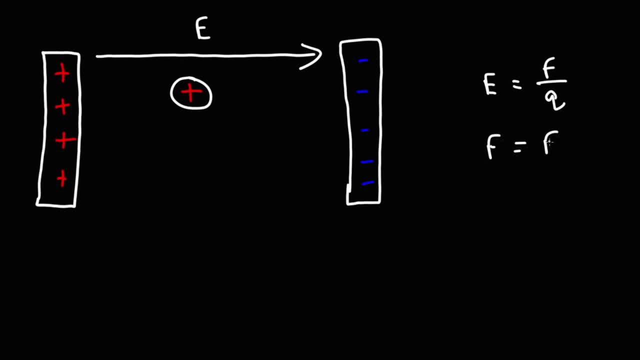 Or, in other words, the electric force is equal to the electric field times the charge. The electric field is a vector and the force is a vector. So this positive charge is going to feel a force that is going to be in the same direction as the electric field. 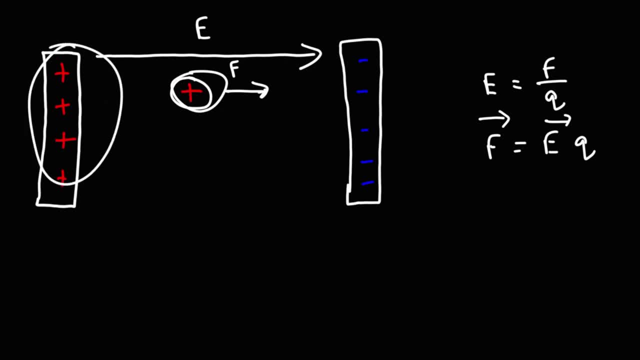 This positive charge is repelled by the positively charged plate, but it's attracted, So the negatively charged plate. So it's going to feel a force, an electric force that's going to accelerate it towards the right. Now, in this example, 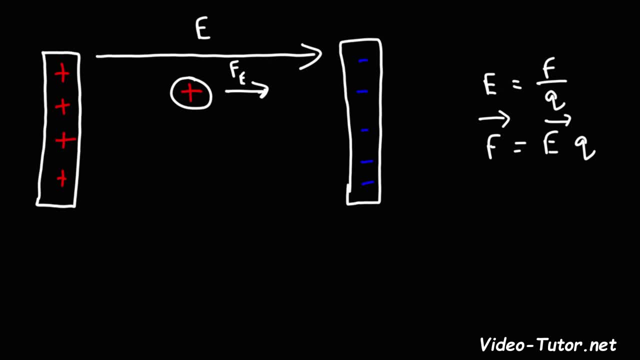 the electric force like gravity and like the restoring force in this spring. the electric force is the conservative force here. Now what's going to happen if we apply a force to move this charge To the left? So we're applying a force that's greater than the electric force. 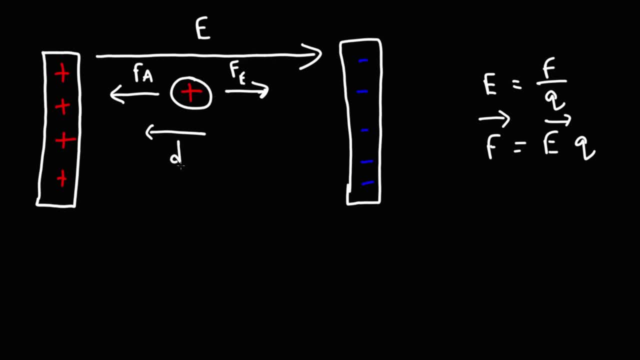 causing the object to move to the left. So what's going to happen to the potential energy of this charge? Is it going to go up or is it going to go down? Because we're moving the charge against the conservative force, against the electric force. 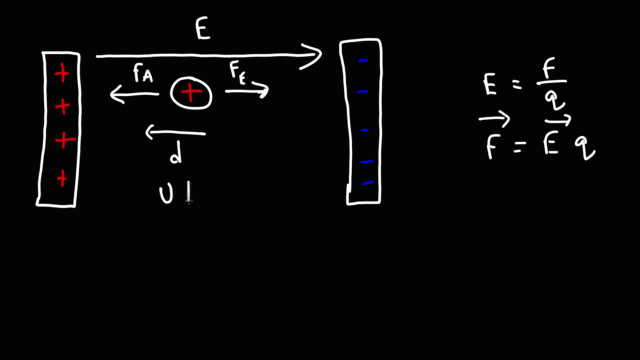 the potential energy is going to increase. These two vectors are opposite to each other. Now, if we were to remove the applied force and if we were to allow the charge to do its thing and allow the electric force to take over, this charge will eventually move in the direction of that electric field. 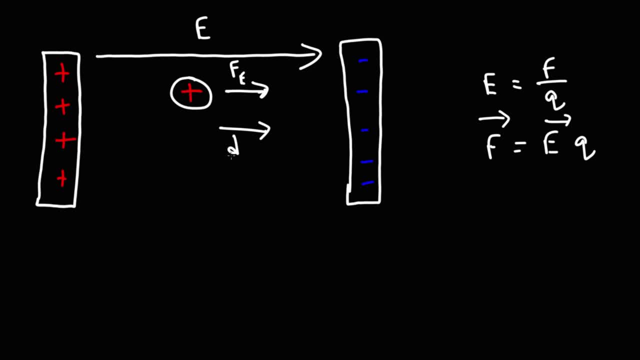 It's going to accelerate in that direction and whether, regardless if it has an initial velocity, at some point, if the field is strong enough, it's going to turn and go towards the right. That's where it wants to go. So, the moment that it's moving to the right, 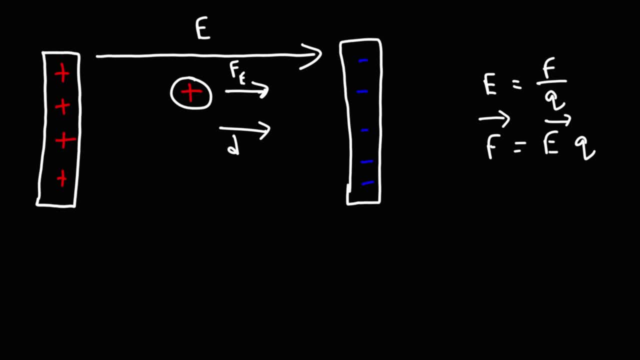 what's happening to the charge? its potential energy? Is it increasing or decreasing? Because the charge is moving in the direction of the conservative force. its potential energy is going to decrease As it moves in the direction of the electric force if there are no other forces acting on it. 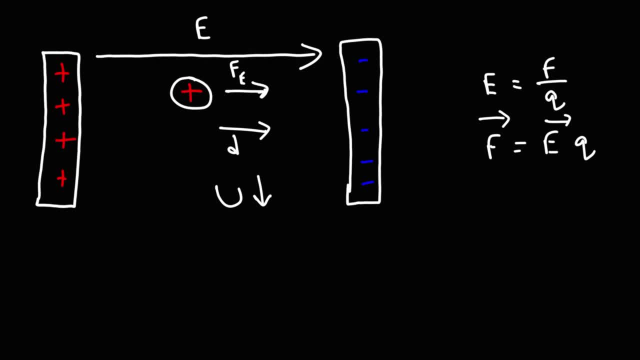 this becomes the net force, and so it's speeding up towards the right, which means its kinetic energy is going up, but its potential energy is going down. So make sure you understand that Whenever you move an object in the direction of the conservative force. 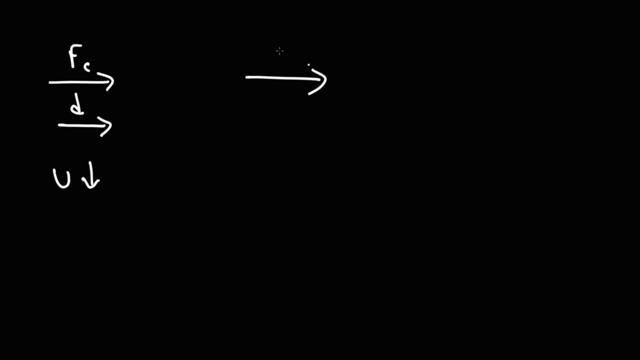 the potential energy of that object decreases. And when you move an object against the conservative force- whether that conservative force is gravity, the restoring force of a spring or the electric force- the potential energy goes up. So I want to make sure you understand. 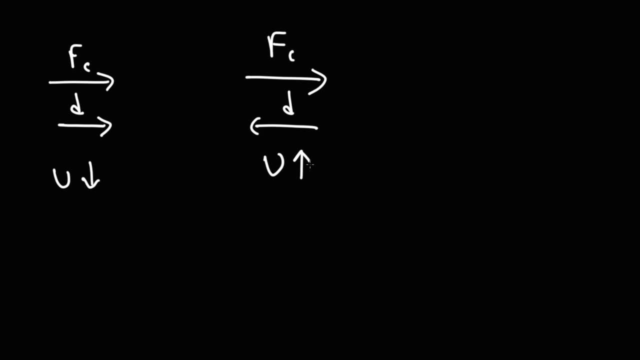 the relationship between force, displacement and potential energy. So notice that the potential energy goes up when they're opposite to each other And it goes down when they're in the same direction. This has to do with the negative sign in this equation. 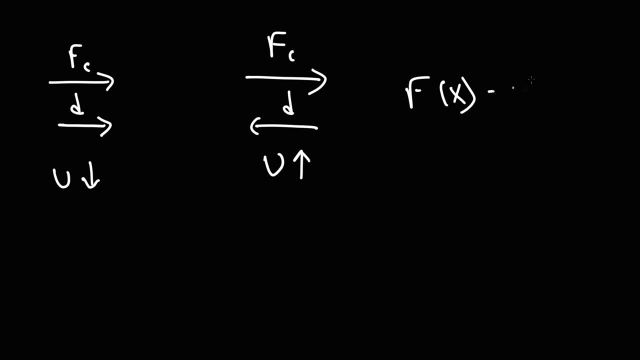 where we know that the force is the negative derivative of potential energy. So because of that negative sign, remember that this is opposite Potential energy. change in potential energy is positive when the vectors are opposite to each other. The change in potential energy is negative. 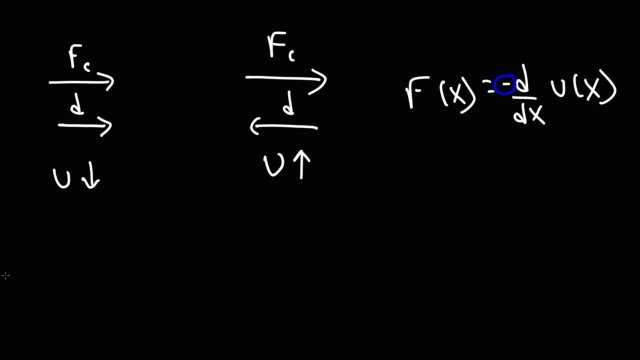 when the vectors are in the same direction with each other. It has to do with this negative sign here. Now let's talk about how we can derive some common formulas. So let's say we have an object with mass m above ground level. So let's say the position of the object. 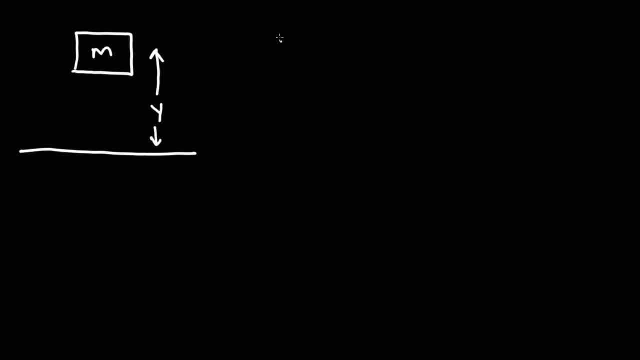 above the ground is y. The potential energy of that object as a function of y is mgy. Now in many other physics textbooks you'll see that the potential energy is mgh. So h and y, you can use them interchangeably. 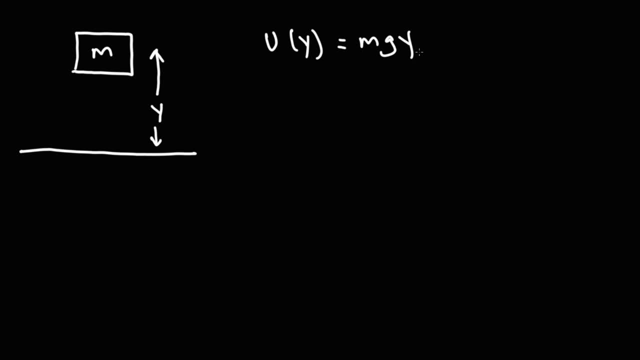 Now what we're going to do is calculate the force function from the potential energy function. Now we know that the force is the negative derivative of the potential energy function. Now this time we're looking for the force in the y direction, So we need to take the derivative. 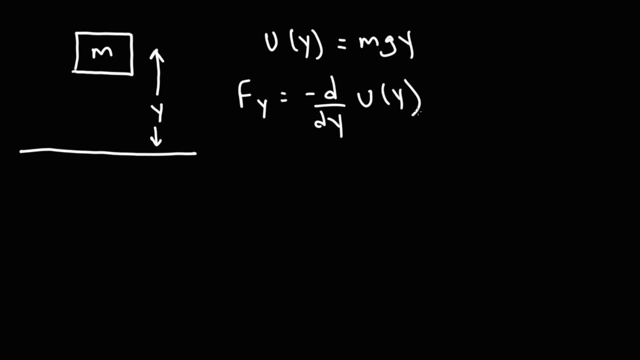 of the potential function with respect to y. So I'm going to replace uy with mg. Now we're differentiating with respect to y, So m and g- anything that's not y- we're going to treat it as constants, So this is going to be negative mg. 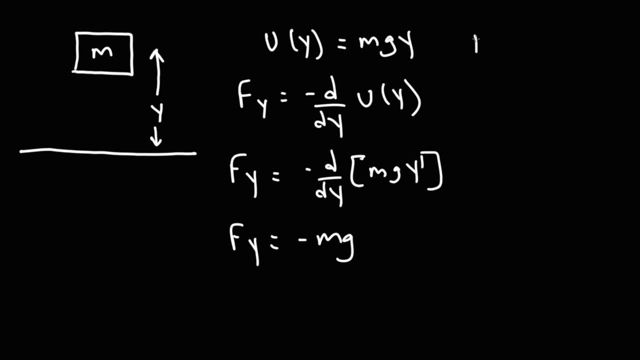 and the derivative of y to the first power. By the way, this is the power rule. The derivative of a variable raised to a constant, x to the n, is going to be nx to the n-1.. So the derivative of a variable, 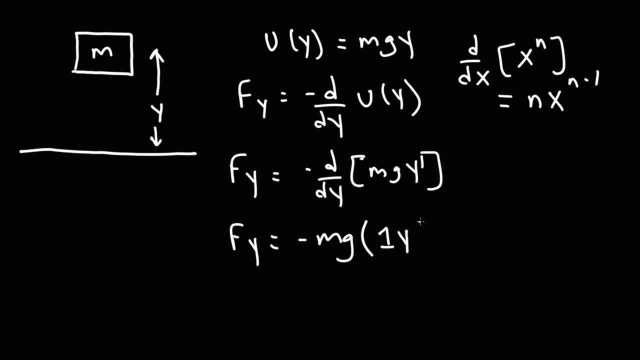 of y to the 1, would be 1y raised to the 1-1, which 1-1 is 0, and anything raised to the 0 power is 1.. So the derivative of y is simply 1.. 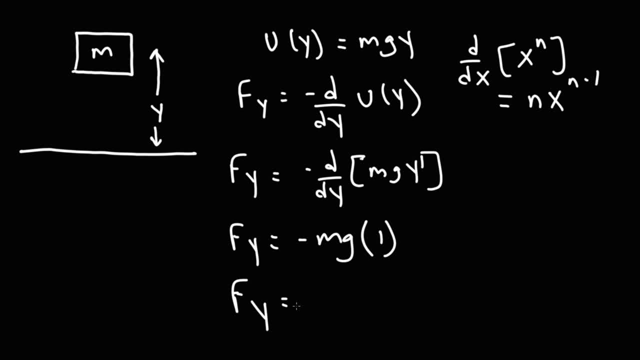 So we get this equation F of y. the force of gravity acting on a mass is simply equal to negative mg, And that makes sense. We know the weight of an object is mg, It's mass times gravitational acceleration, Very similar to the sense that the lift force. 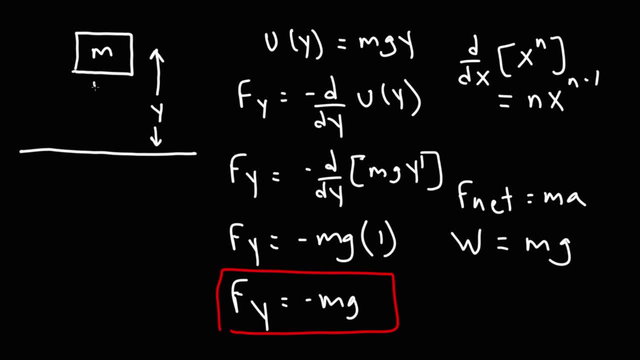 is ma And the gravitational force is in the negative y direction. So we could see the negative sign here, Because if m is positive and g is positive, then we need to introduce a negative sign, such that we get a negative vector or a vector point in the negative y direction. 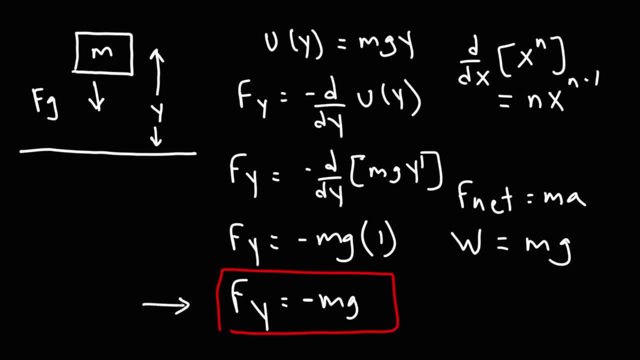 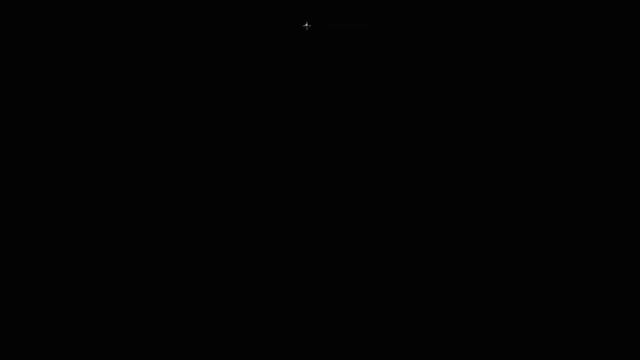 So that's it. So that's how you can get the weight force equation, or gravity, from the potential energy equation. Now let's move on to springs. So let's say we have a compressed spring, just like before, And let's say this is: 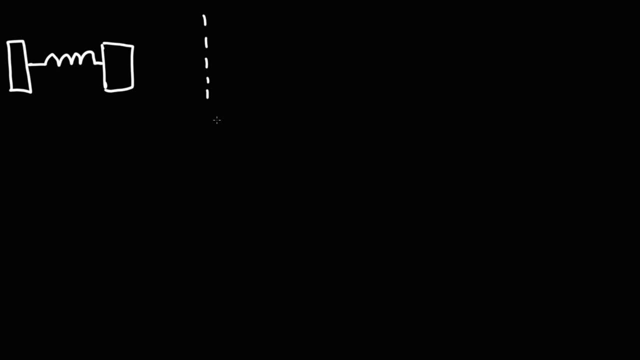 its natural position. This is going to be x. x is the distance between the center point and where the object is currently located, And we know the restoring force is going to be directed towards the point of equilibrium, the center. Now the potential. 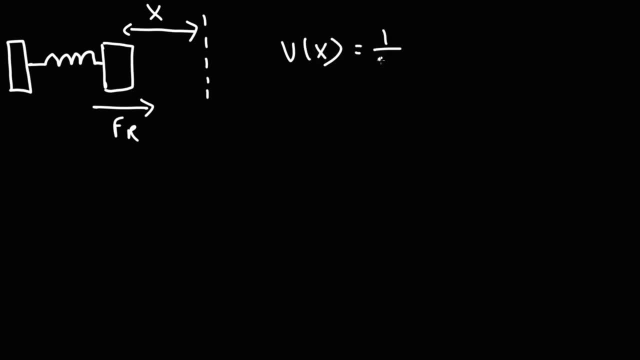 energy function for spring is going to be 1, half h- x squared. Let's calculate the force function from the potential energy function. So we know the force function f of x is going to be the negative derivative of the potential energy function. So that's. 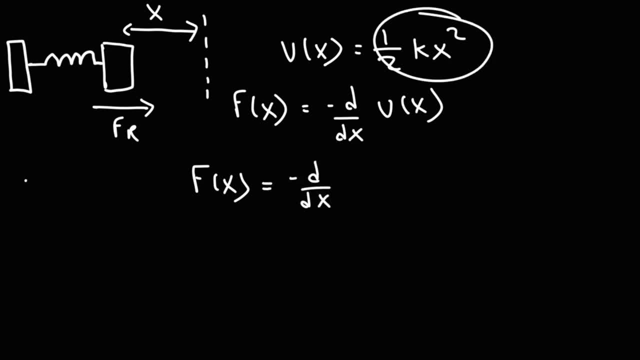 negative d dx of this equation. So the 1 half and k are constants. So I'm just going to rewrite them. So we have 1 half k and now we need to find the derivative of x squared. So using this formula: 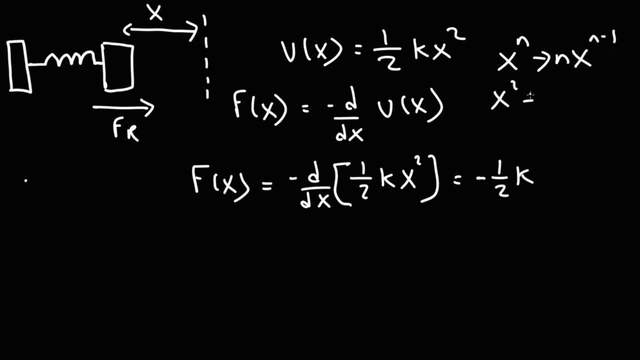 it's going to be n is 2, so it's 2 x to the 2 minus 1, or 2 x to the first power, or simply 2 x, Now 1 half times 2 x 1 half times 2 is 1.. 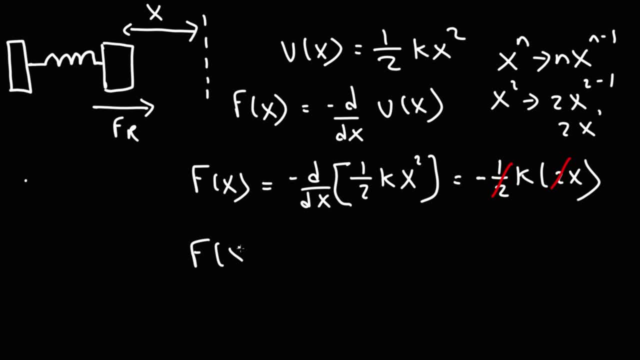 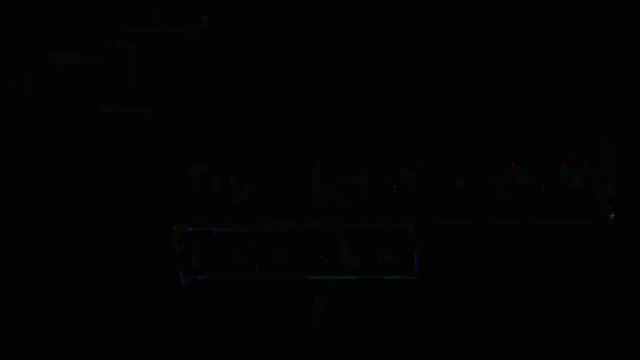 So we get this equation: f of x is equal to negative f, k, f. So this equation gives us the magnitude of the restoring force. And let's see how the negative sign plays a role in this equation. Let's undo that. So at the center point, 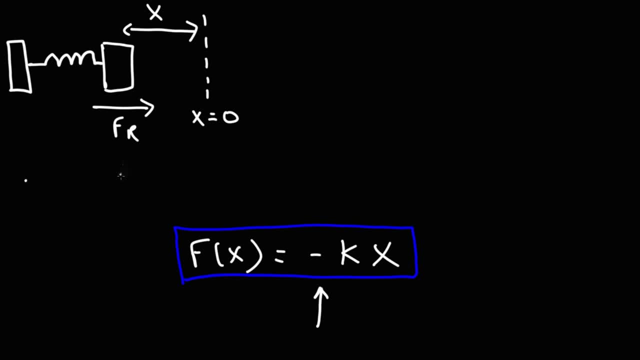 x is 0.. At this position, where the object is located, it's to the left of the x equals 0 point, Which means, at this position, x is negative. Now, if x is negative in this equation, what's going to be the sign of f? 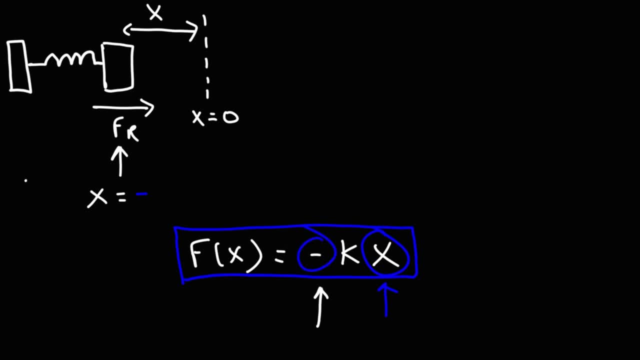 So this is negative times, another negative. Two negatives make a positive. The restoring force is going to be positive, And we can see that When the spring is to the left of the equilibrium point, the restoring force is directed towards the right, And so it's positive. 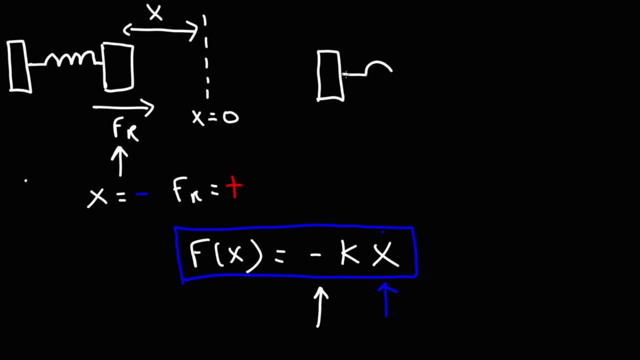 Now if we were to draw the other scenario, let's say, if we expand the spring above its natural point, if at this location x is 0, at this point x is going to be positive. The restoring force is going to be directed to the. 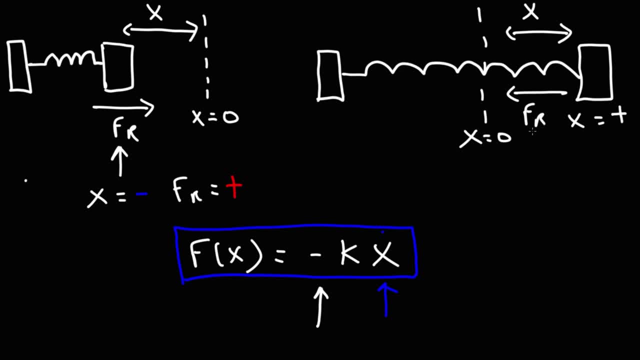 left, The spring will want to compress back to its equal in position. Now, if x is positive and we multiply it by a negative sign, a negative times a positive will give us a negative result. That means that the restoring force is going to be. 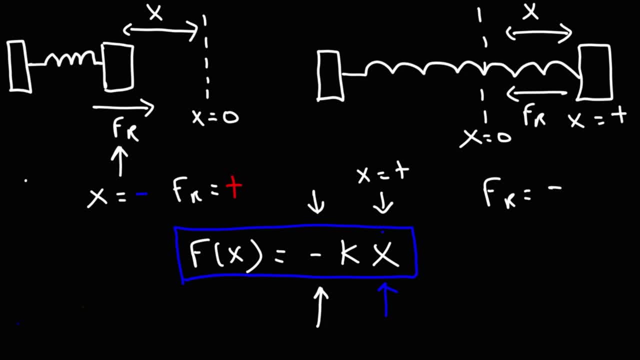 negative, Which in this case it is. Once you dredge the spring beyond its natural length, the restoring force wants to bring the spring back to the left, And so we can see why we have the negative sign. So this equation not only tells you the magnitude. 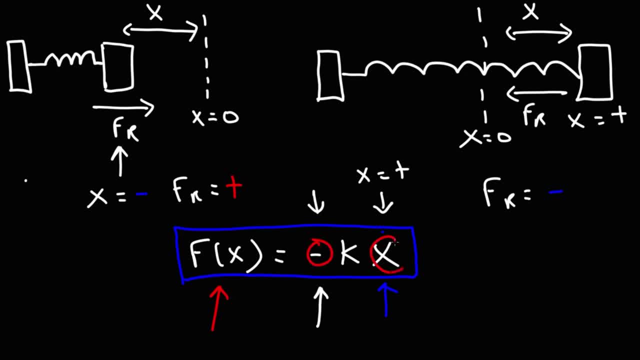 of the restoring force, but when you incorporate the appropriate signs you also can determine the direction of that force from this equation And of course you can figure it out intuitively if you draw a picture. But at least now you know how to get this equation. 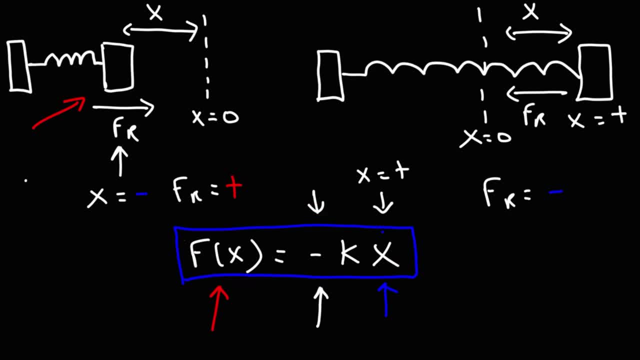 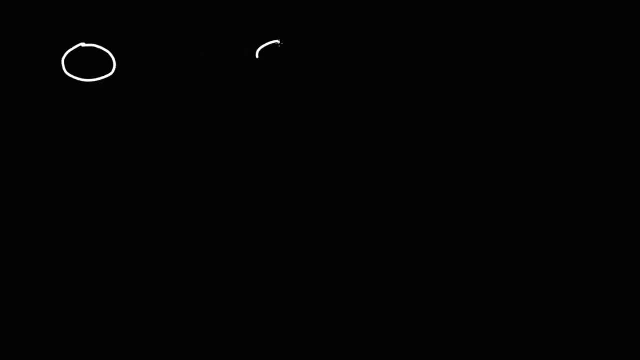 from the potential energy equation of a spring. Now let's say, if we have two charges, and let's say that both charges are positive, the magnitude of this charge is q1, and for this one it's q2.. And the distance between 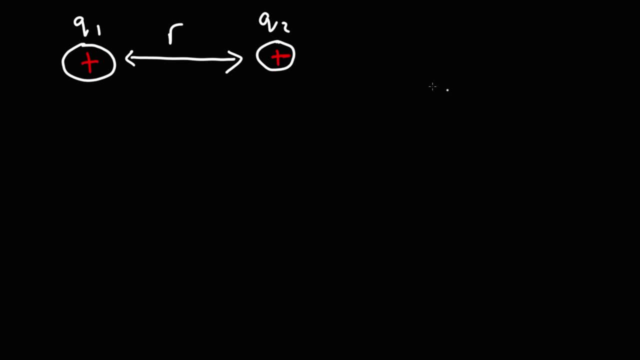 them. we'll call it r Now the potential energy function between two charges. it depends on the variable r. It's equal to k, which is a constant. it's like 9 times 10 to the 9, times the magnitudes of q1 and. 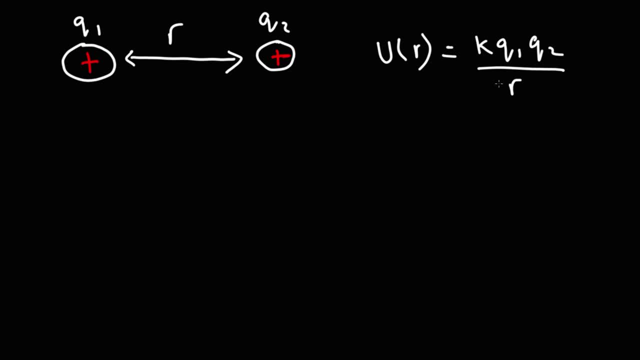 q2, divided by r. Let's get the force function from this potential energy function. So the force function as a function of r is going to be negative d dr of the potential energy function. So we're going to find the derivative of this function. 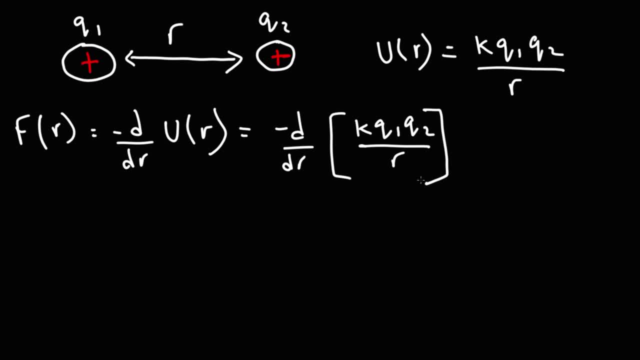 with respect to r, Because k, q1, q2, they're all constants in this equation, The electric charge, q1 and q2, they're fixed values and k is a constant. So the only thing that we can really 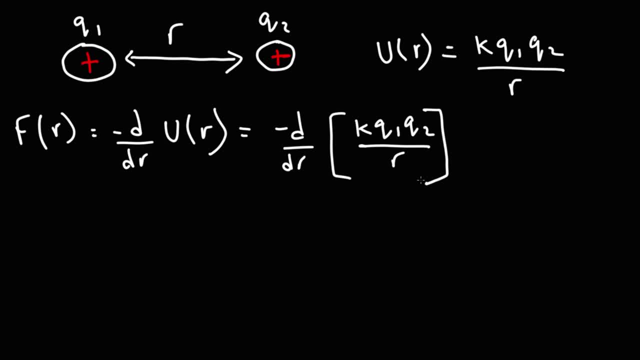 vary is the distance between the two charges. Now, using the power rule for derivatives, we have this equation. So let's take the derivative of 1 over r. By the way, I'm going to rewrite this as negative d dr. I'm going to. 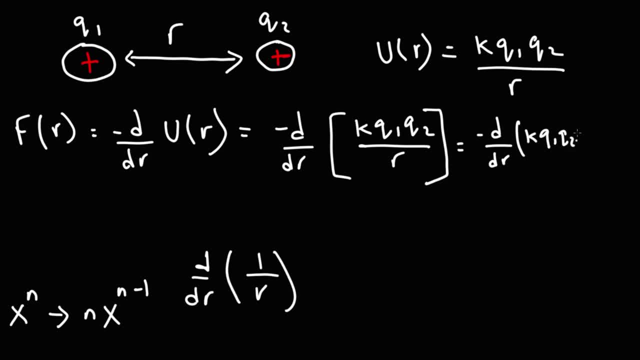 separate the constants k, q1,, q2, and then this is multiplied by 1 over r. So now I'm going to focus on differentiating just the variable part. If we move the r to the top, this becomes r. 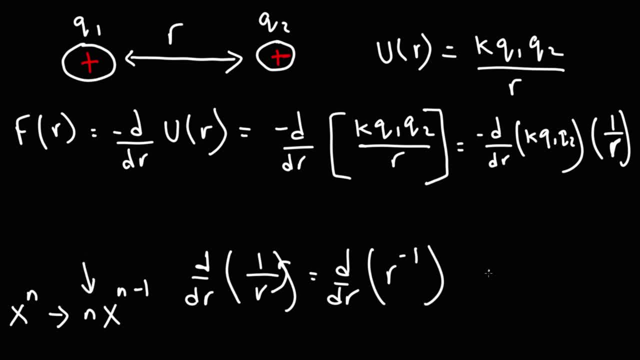 negative 1.. So in this equation n is negative 1. So this becomes negative 1 times r raised to the negative 1 minus 1.. Which becomes negative r minus 2.. And if we put this over 1 and bring the r back down, 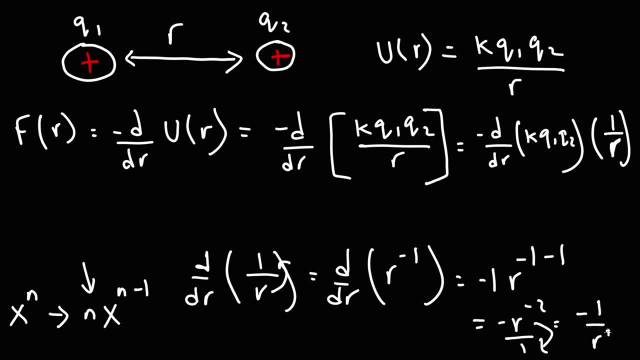 the negative exponent will become positive. so we get negative 1 over r squared. So that is the derivative of 1 over r. It's negative 1 over r squared. So now that we've applied the derivative function, we can get rid of this. 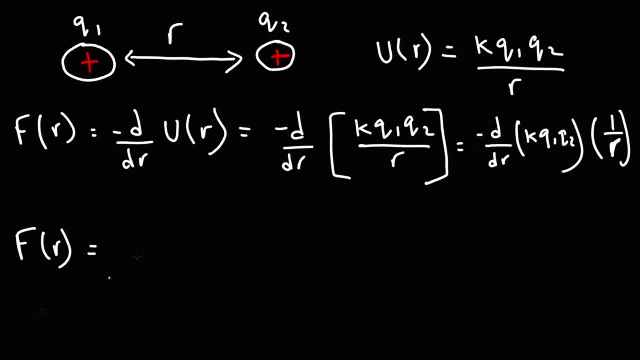 But we still have the negative sign. So we have a negative and then we have k, q1,, q2, and then the derivative of 1 over r we said was negative: 1 over r squared. Now the two negative signs will cancel. 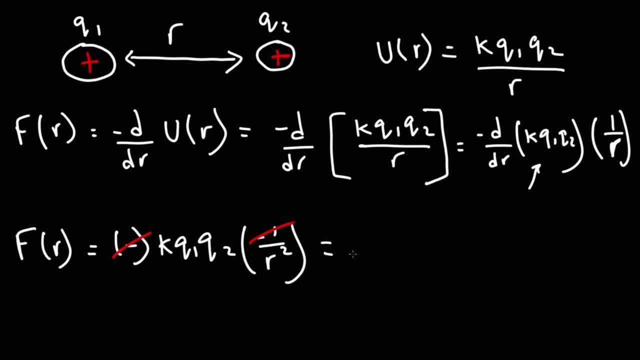 And so now we're going to have the equation that will give us the electric force between two charges, which is k, q1, q2 over r squared. So that's how you could derive this equation from the potential energy function of two charges. 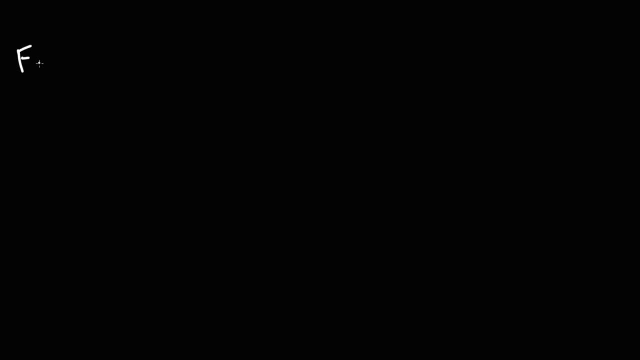 Now here are some other things you want to know when dealing with force and potential energy. The component of the force in the x direction can be calculated by measuring the change in potential energy as the object moves along the x direction. Now the component of the force. 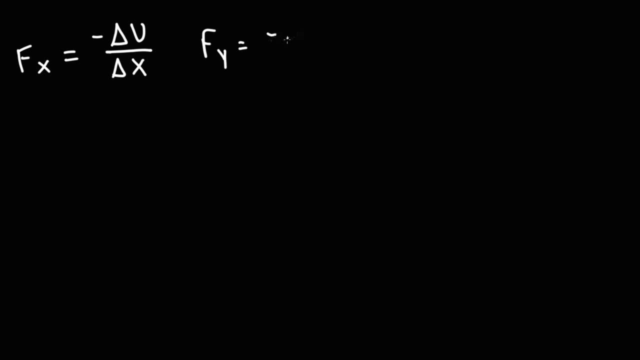 in the y direction. you can also calculate that by measuring the change in potential energy that the object experiences when moving along the y direction, And you can also do that in the z direction as well. So what this means is that the x component 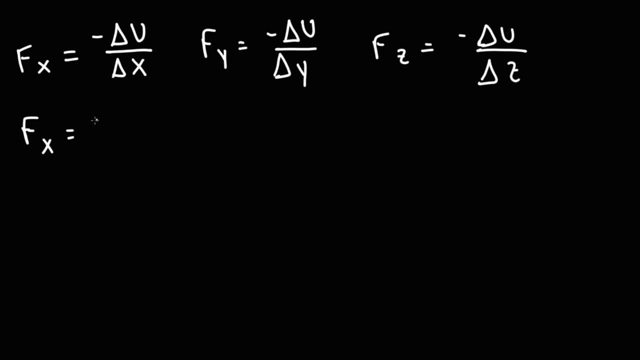 of the force is equal to the negative partial derivative of the potential energy function with respect to x. The y component of the force is equal to the partial derivative of the potential energy function with respect to y, And the same is true for the z component of. 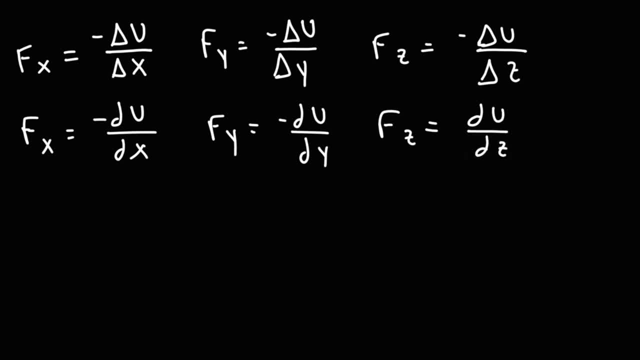 the force. So what we've been doing is we've been calculating the partial derivative of the potential energy function with respect to the different coordinates, such as x, y and z. So this operation, the operation that, when we take the partial derivative of the potential energy function, 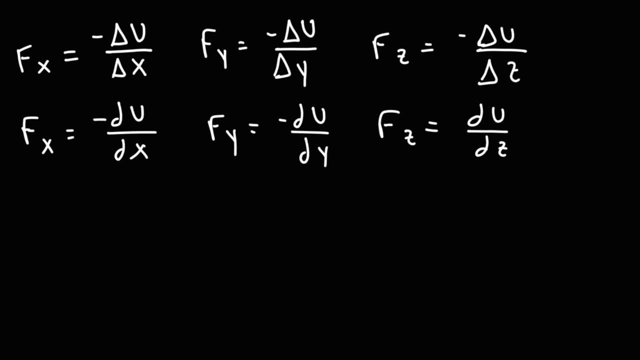 with respect to each coordinate. this will help us define what is known as the gradient of u. So we can write the force vector like this. So the force vector is going to be negative times. the partial derivative of the potential energy function in the x direction. 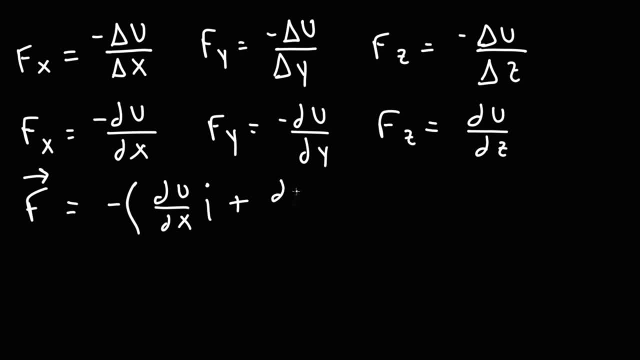 times the unit vector i, plus the partial derivative of the potential energy function with respect to y times the unit vector j, plus the partial derivative of the potential energy function with respect to z times the unit vector k. So when we take the partial derivative of the potential energy, 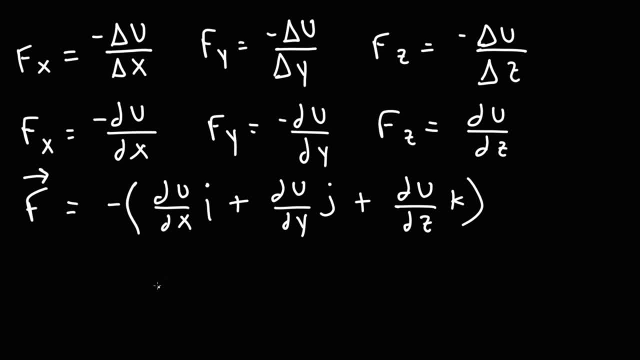 function. with respect to each of these coordinates, we now have what is known as the gradient. So force is the negative gradient of the potential energy function. So that is a special operation of derivatives. So that's something you may want to add to your notes. Force is the negative. 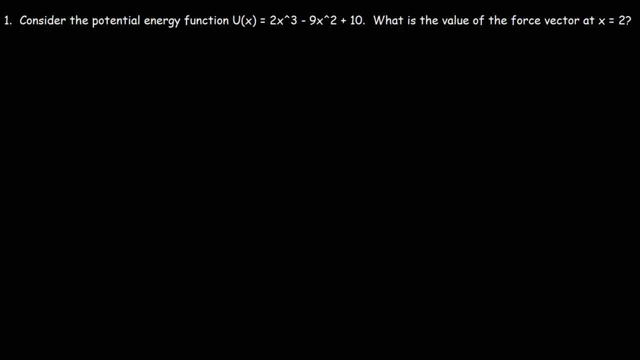 gradient of the potential energy function. Now let's work on a practice problem. Consider the potential energy function. ux is equal to 2x, to the third power, minus 9x, squared plus 10.. What is the value of the force vector at x equal 2?? 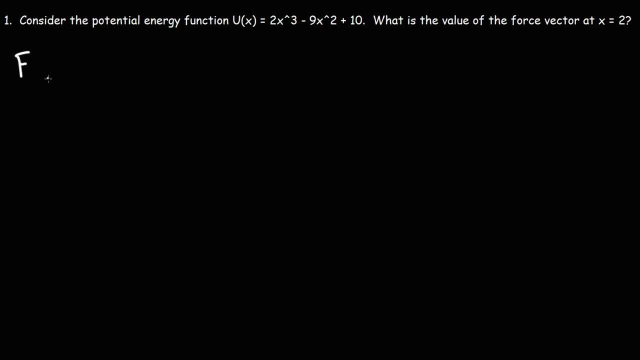 Well, the first thing we need to do in this problem- By the way, feel free to pause the video if you want to try this- The first thing we need to do is calculate the force function. We know the force function is the negative derivative. 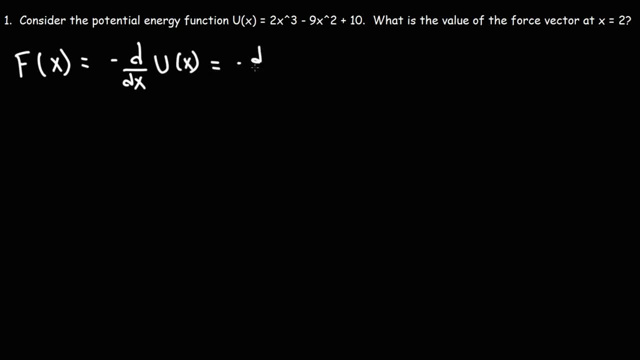 of the potential energy function. So we have negative ddx of 2 x cube minus 9x squared plus 10.. The derivative of x cube using the power rule x to the n is nx to the n minus 1.. By the way, for those of you who 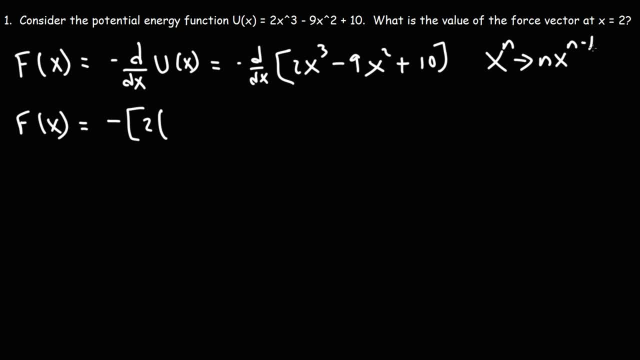 want some more practice on that. I have a video entitled Power Rule on Derivatives. If you look that up on YouTube and if you type in Organic Chemistry Tutor, that video should come up. so you'll know how to find the derivative of functions. 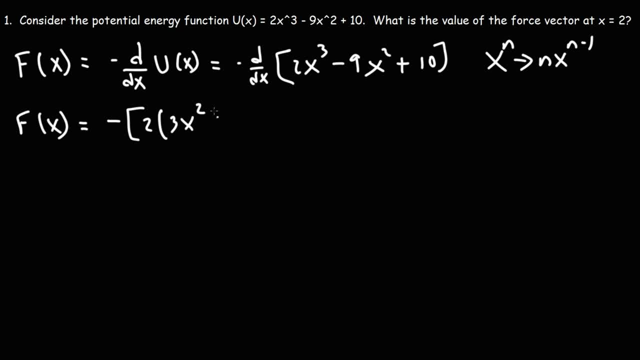 But the derivative of x cube is going to be 3x squared And the derivative of 2x is going to be 2x to the first power, which is simply 2x, And the derivative of any constant is 0.. 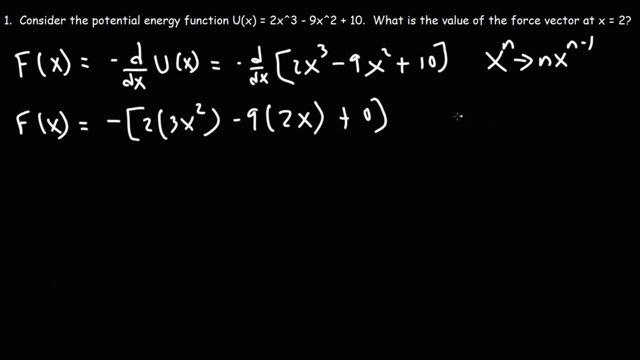 If you want to use that formula to find the derivative of a constant view, 10 as being 10 times x to the 0. Because x to the 0 is 1.. And so this becomes 10 times 0 x to the 0. 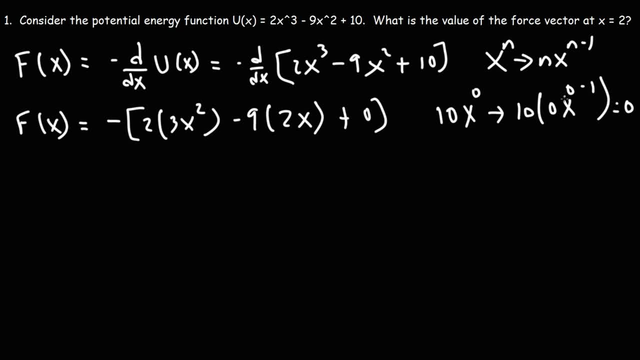 minus 1.. 0 times anything is 0. So even if you were to use that formula, you would still get the right answer: Constants. So this becomes negative: 6 x squared plus 18x. Don't forget that we have two negative signs here. 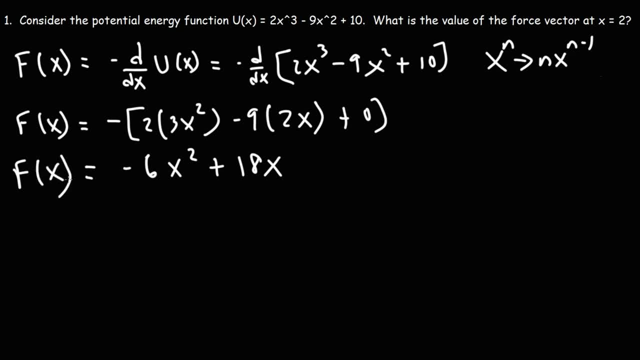 So that's going to be the value of the force function with respect to x. So now we're going to find the value of the force function when x is 2.. So we have negative 6 times 4 plus 36.. So that's negative 24. 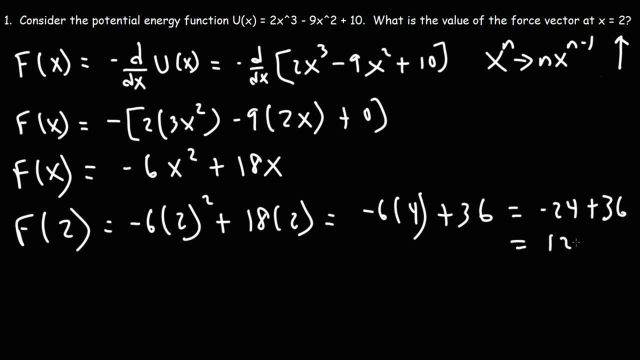 plus 36, which is positive 12.. So the force vector is going to be 12. i So, because we were finding the derivative with respect to x, the force is going to be in the x direction. So this is basically the component of the force in the 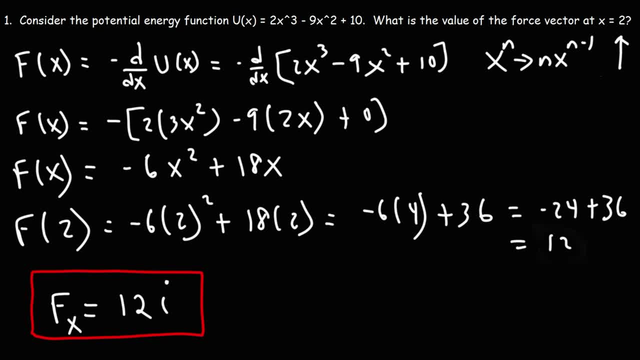 x direction And we have a value of 12.. And because it's positive, we know the force is along the positive x direction, So it's going to the right. So we have the magnitude of this component force, which is 12.. And we have 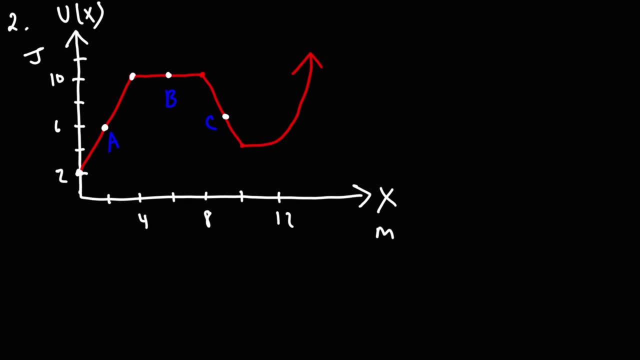 the direction, which is to the right or east. Now let's move on to number 2.. So here we have a graph of the potential energy as a function of x. On the y-axis. the potential energy is measured in joules On the x-axis. 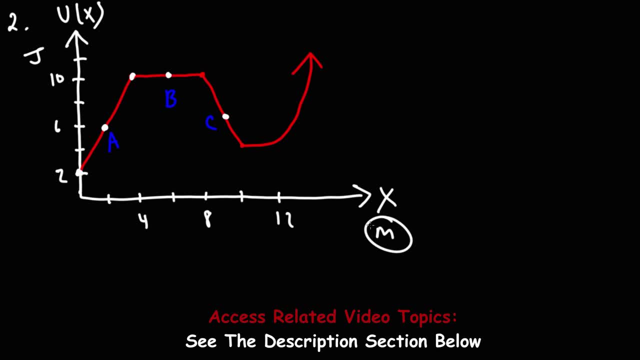 the position is going to be along the x direction, but the unit is in meters. With this information, calculate the value of the force vector by points A, B and C. Now we know that the force, the x component of the force, 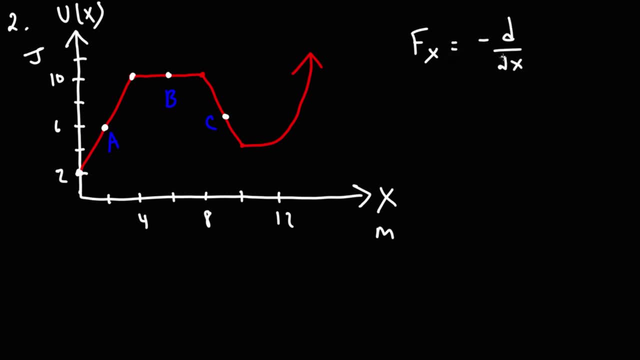 is going to be the negative derivative of the potential energy as a function of x, And the value of any derivative function is equal to the slope of the tangent line. So we can calculate the value of the force by calculating the slopes of the graph at points. 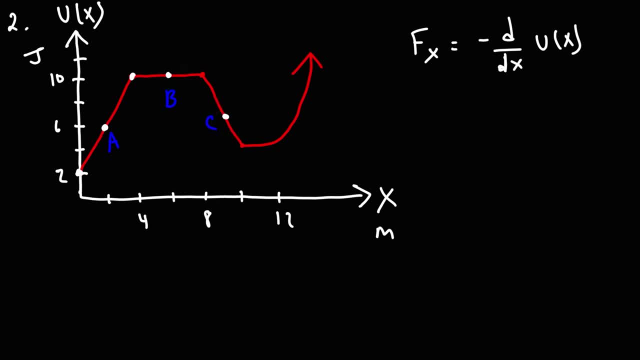 A, B and C. Now we know that slope is rise over run, So you could use this formula to get the answer, but you need to be careful. You need to incorporate this negative sign. So f of x is going to be. 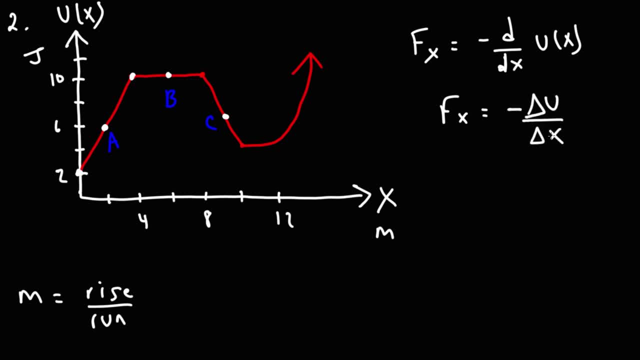 negative delta u over delta x. So this is similar to the slope function, where for the slope function we have a change in y over the change in x, but instead of the change in y we have the change in u And delta x is the same. but 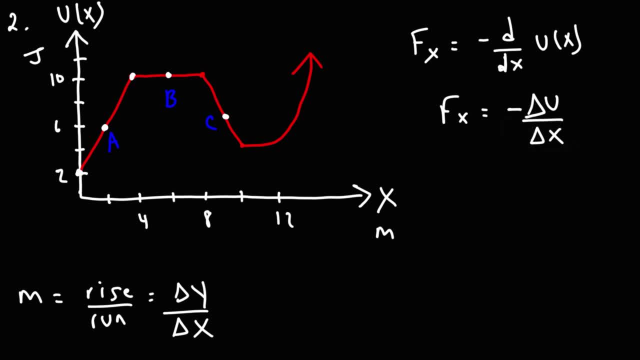 we need to incorporate the negative sign. So that's what you have to be mindful here. So let's calculate the slope of the tangent line at point A, which is the slope of the secant line or that segment. So at point A, 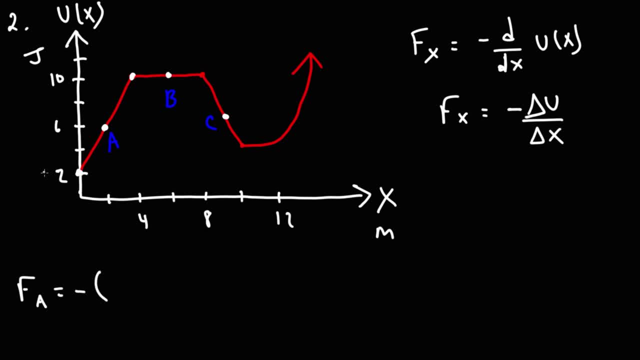 notice that we have a rise of 8.. So, going from- if we focus on these two points here, we're going up 8 units and then the run, we're going to the right 4 units. So that's a rise of 8, a run of 4.. 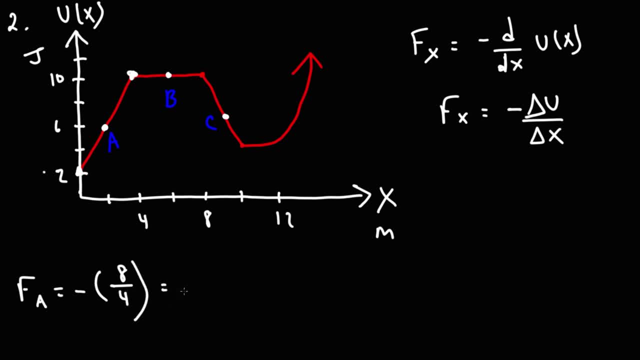 That will give us a slope of positive 2. Because we need to multiply it by a negative sign, we get negative 2. So at point A the force is negative. So we can say that F of A is negative 2 newtons. 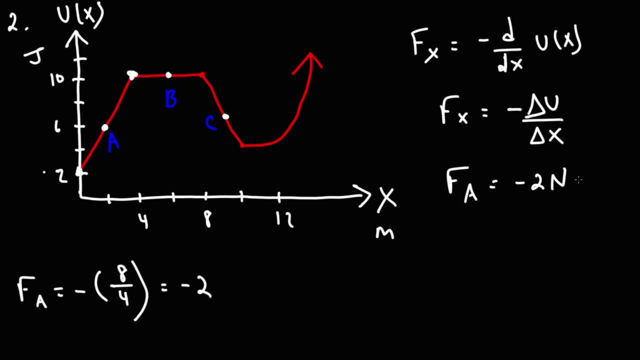 and because we took it along, we differentiated the potential energy function with respect to x. this is the x component of that force. So F of A is negative, 2 newtons times the unit vector i. So because it's negative, that tells us: 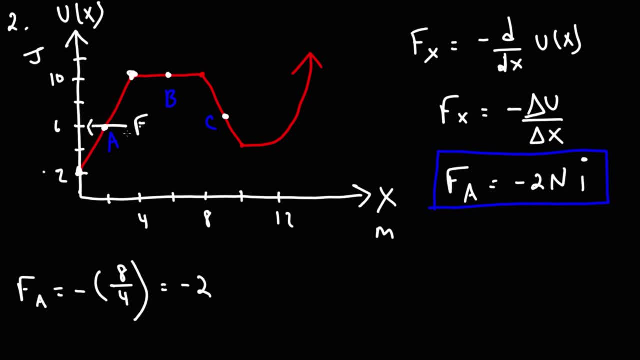 that the force at point A is directed the left. Now what about at point B? Notice that we have a horizontal tangent line at point B, And the slope of any horizontal line is 0, so F of B is just going to be 0.. 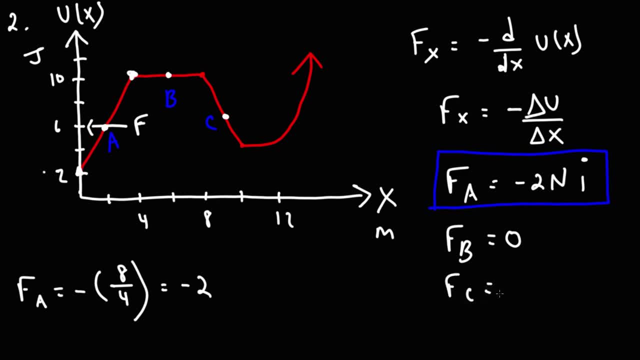 Now what about F of C? So F of C is going to be negative. notice that the rise we're going from, if we focus on these two points, we're going from 10 to approximately 4, so that's a rise of negative 6.. 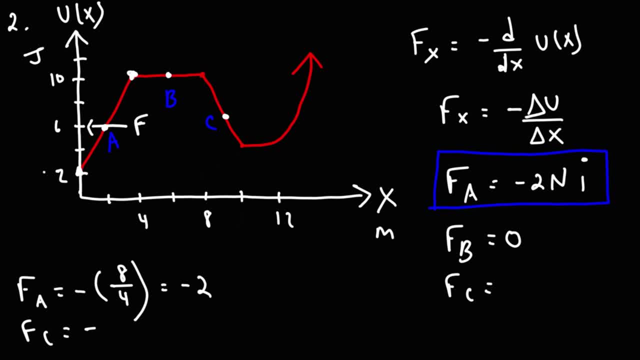 And here we're going from 8 to 10,, so that's a run of 2.. So we have negative and then a rise of negative 6, divided by a run of 2. So the two negatives will cancel out. 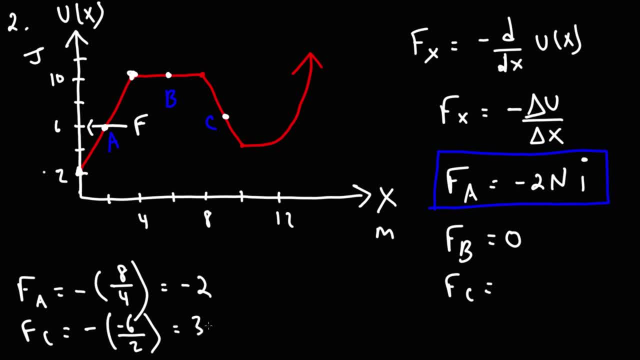 we get that the force is 3.. So the slope is negative: 3,. this line has a negative slope. the force is positive. So F of C is going to be positive, 3 newtons times unit vector I, since we're still 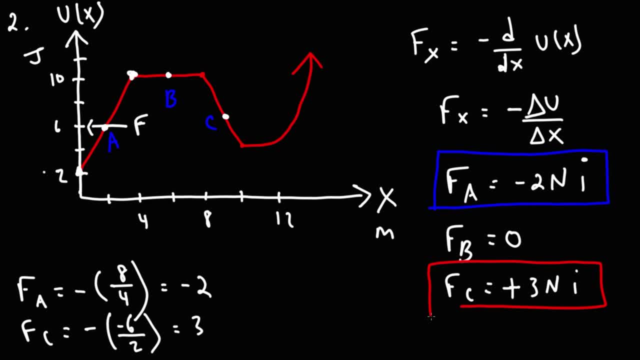 differentiating it with respect to x. So because the force is positive, it's going to be pointing towards positive x direction. So now let's summarize what we're learning here In this segment, as we go from 0 to 4 in the x direction. 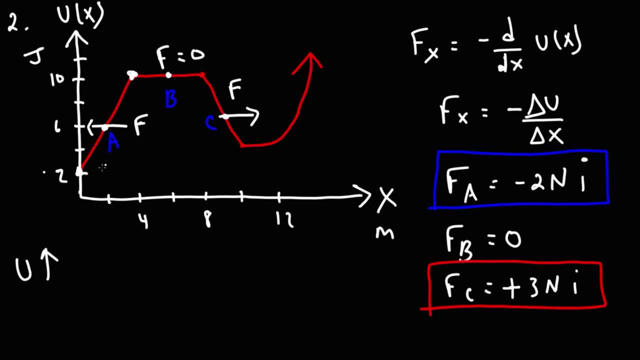 the potential energy is increasing because we're going up. So the potential energy is increasing as we move to the right, but the force is negative. So the force is in the opposite direction, It's to the left. And remember what we said earlier. 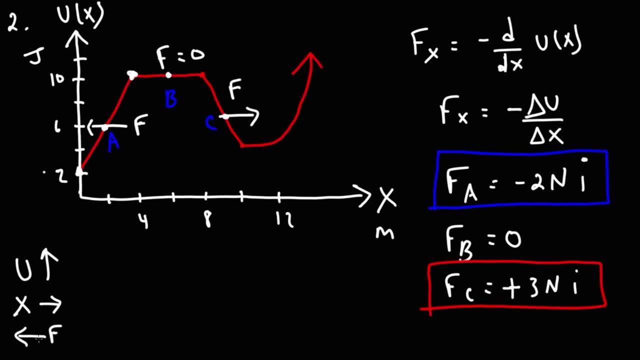 that whenever an object moves in the direction opposite to the conservative force, the potential energy increases And we can see that The displacement and the conservative force vectors. they're opposite to each other, So the potential energy is going up In this segment. 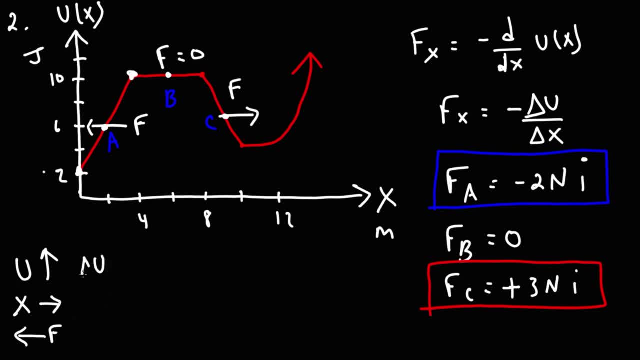 the potential energy is constant, So the change in potential energy is 0.. We're still moving to the right, but there's going to be no force. So if an object is moving in a direction where there is no conservative force, there's going to be no change. 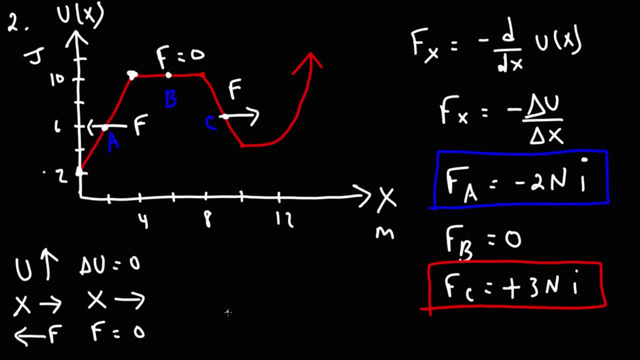 in potential energy. So this could mean there's no conservative force or no force acting in the x direction. A good example of that is, let's say, if you have a block and you move the object along the x direction, Now the force of gravity. 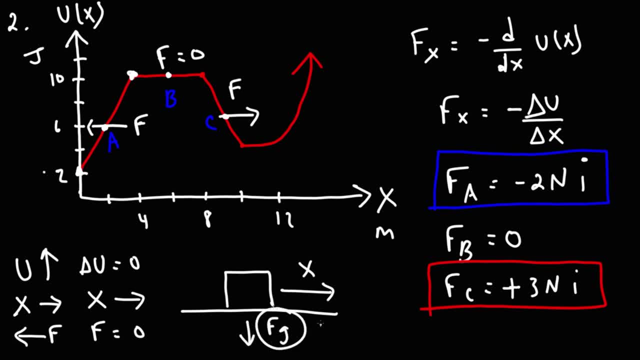 is in the y direction. This conservative force is not parallel to the x direction, And so as you move the object to the left or to the right, there's going to be no change in potential energy of that object with respect to gravity. Now let me try explaining. 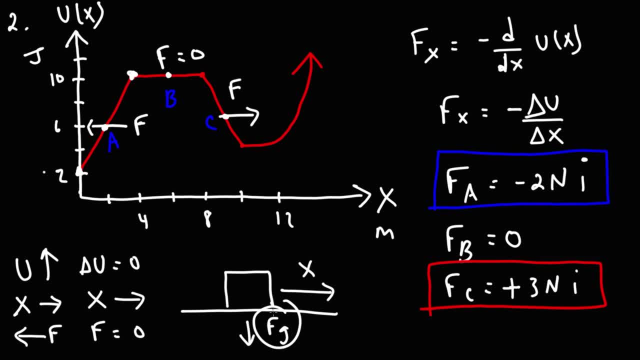 this another way. The force of gravity acting on this object is not zero. It has a value, And that is. it has a value in the y direction. It is zero in the x direction. The force of gravity has no value in the x direction. 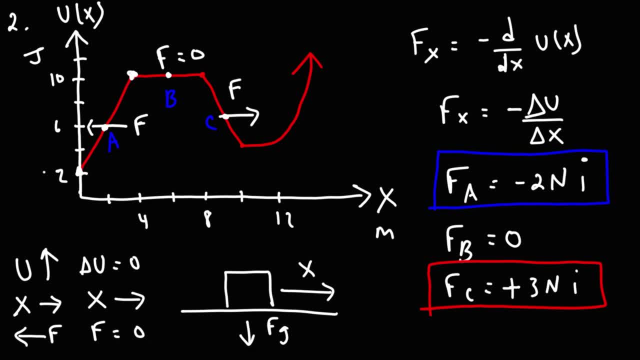 for this particular situation, And so, because the conservative force in the x direction is zero, you can move along the x axis whether to the right or to the left. there is no change in potential energy with respect to the gravitational force, Because there is no gravitational force. 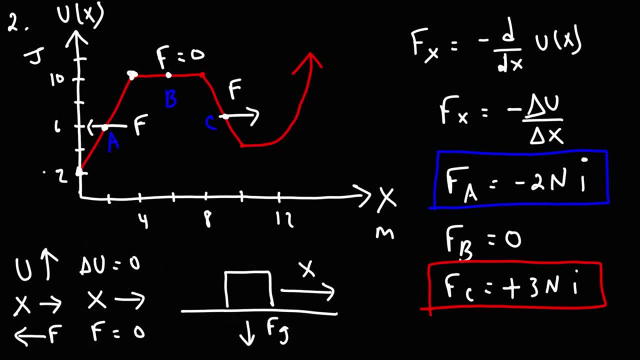 in the x direction It's equal to zero. So in the absence of the conservative force, an object that moves will have no change in potential energy if there is no conservative force. Now let's look at part c In this segment: potential energy. 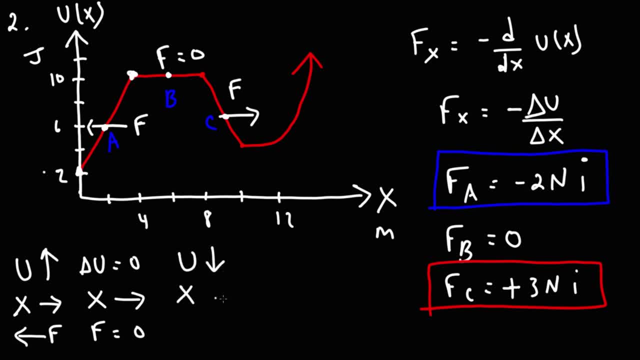 is decreasing because the slope is negative. It's decreasing as we move to the right along the positive x axis. Now the force is to the right, so the force is positive And this agrees with what we said earlier. Whenever an object moves in the direction. 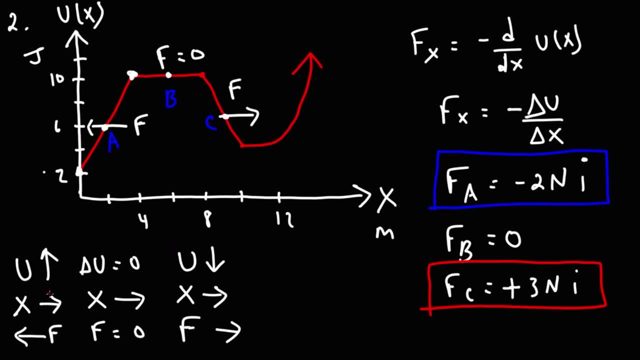 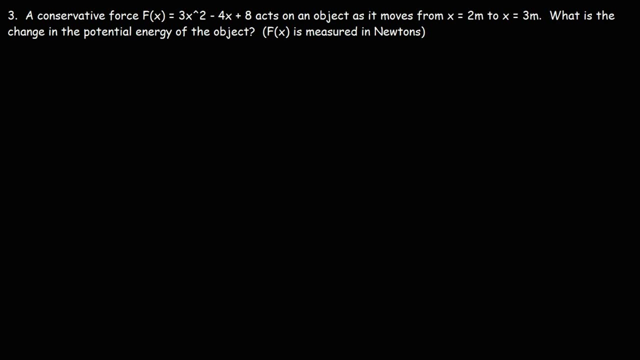 of a conservative force, the energy will decrease, And when the object moves in the direction opposite to the conservative force, the potential energy increases. Number three: A conservative force f of x equal to 3x squared minus 4x plus 8. 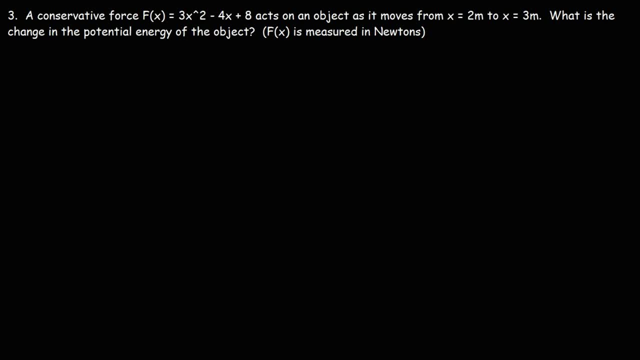 acts on an object as it moves from x equal 2 to x equal 3 meters. What is the change in the potential energy of the object? Now we know that the force in the x direction is the negative derivative of the potential energy function. 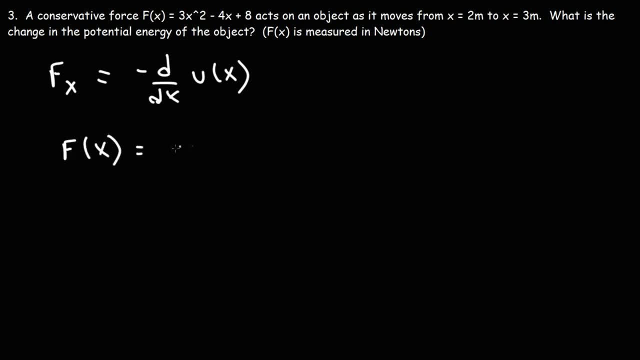 In other words, we could say that f of x is equal to negative u prime of x. This is another way of representing derivatives. If we multiply both sides by dx, we'll have this. And then if we integrate both sides on the left, I'll just keep. 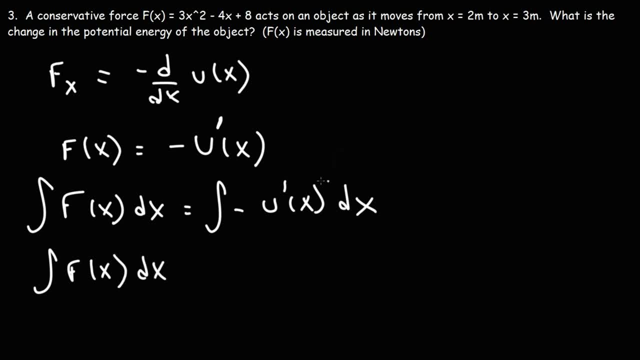 it the same On the right. the anti-derivative of u prime is simply u, So this becomes negative, the potential energy function. So, multiplying both sides by negative 1, we get that the potential energy function is the negative integral of the force function. 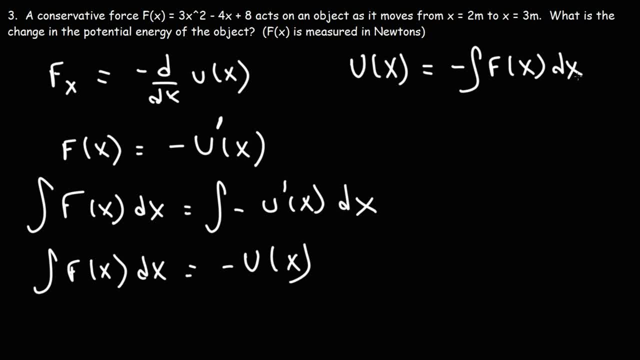 Which also means that if you have a graph of the force function with respect to x, the area under the curve will give you the change in the potential energy function. Either way, in order for this to work, you need to add plus c. 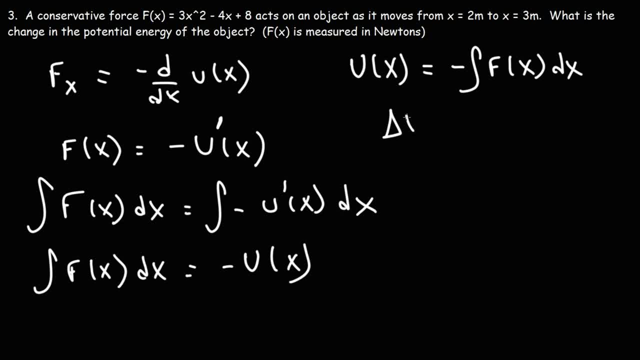 If you don't have plus c, then what you get is the change in potential energy if you were to integrate it from a to b. So if you were to calculate the definite integral from a to b, that will give you the change in potential energy. 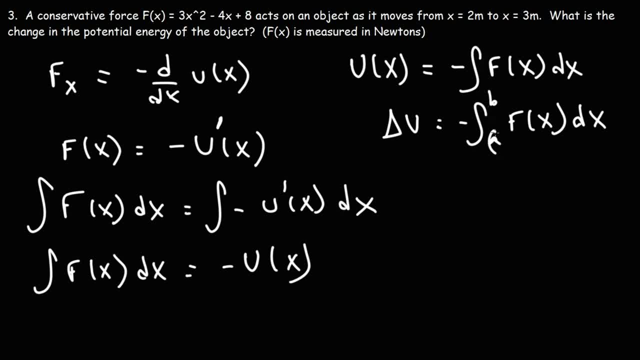 But if you were to calculate the indefinite integral, where you don't have a lower and upper limit of integration, this will give you the potential energy function as long as you evaluate or find the value of the constant of integration. So make sure you understand the difference between the two. 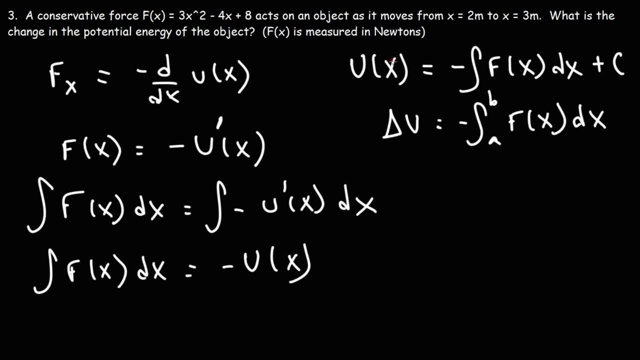 If you want to calculate the potential energy function from the force function, you need to find the indefinite integral of f. If you want to calculate the change in potential energy, which is what we want to do, you need to find the value of the definite integral. 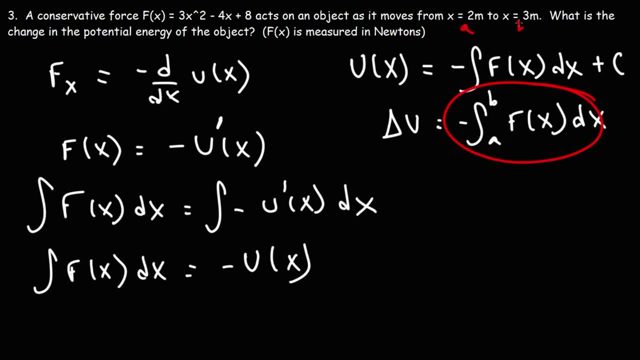 Which, in this case, we have the value of the lower and the upper limit of integration. So let's begin. Delta u is going to be negative of the integral from 2 to 3.. And we have f of x, so f of x is 3. 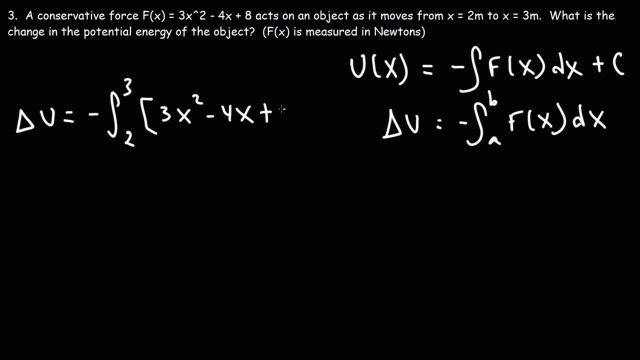 x squared minus 4x plus 8 times d x. Now, if you want to use the power rule for integration, here's how it works: You need to add 1 to n and then divide by that result, So the antiderivative. 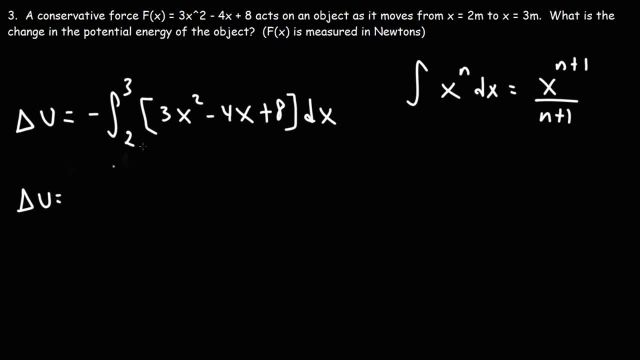 of x squared is going to be: we're going to add 1 to 2, which is 3, and then divide by that result. For x to the first power, it's going to be x squared divided by 2.. And for a constant. 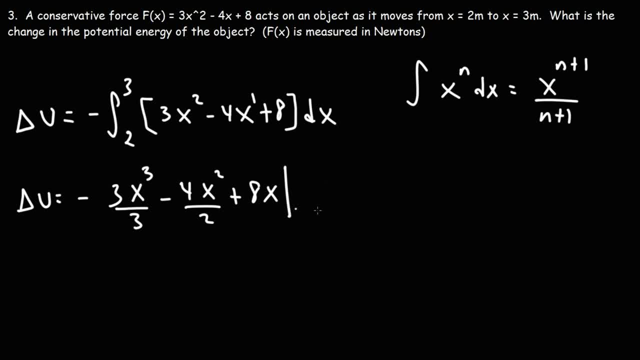 we just simply add an x to it And we're going to evaluate this from 2 to 3.. For those of you who are not familiar with this, I recommend looking up the videos: Definite Integrals- Organic Chemistry Tutor. If you put that into the YouTube search bar, 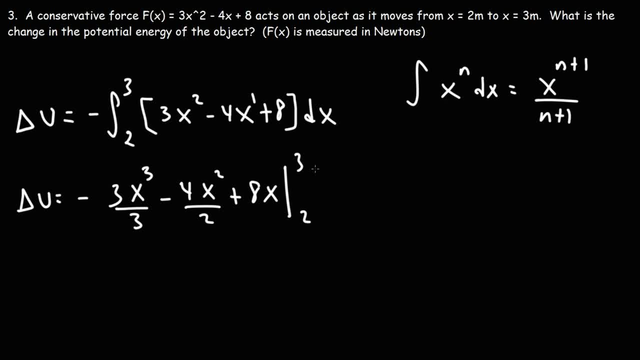 you'll get more examples on how to evaluate definite integrals. So the first thing we're going to do is let's take this negative sign out in the front. We're going to plug in the top number into what we have here, But let's. 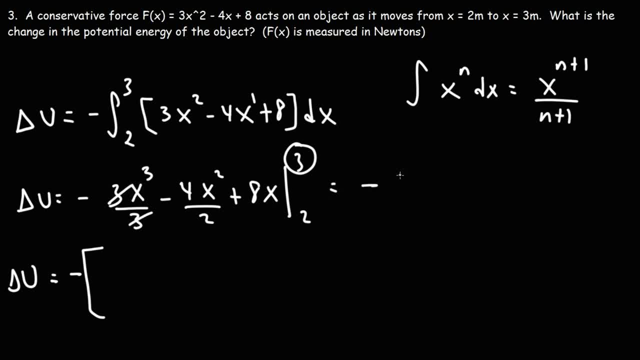 simplify this expression So we can cancel the 3.. Thus we have x cubed Negative. 4 divided by 2 is negative 2.. And then we have 8x evaluated from 2 to 3. So first we're going to plug in 3.. 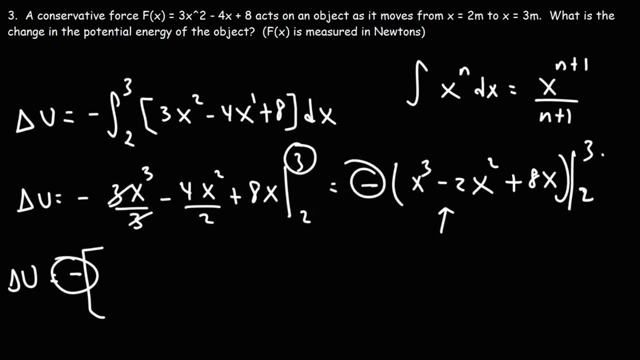 And I've moved the negative sign to the outside here. So this is going to be 3 to the third power minus 2 times 3, squared, plus 8 times 3 and then minus. now we're going to plug in 2.. So this is 2 to the third power minus. 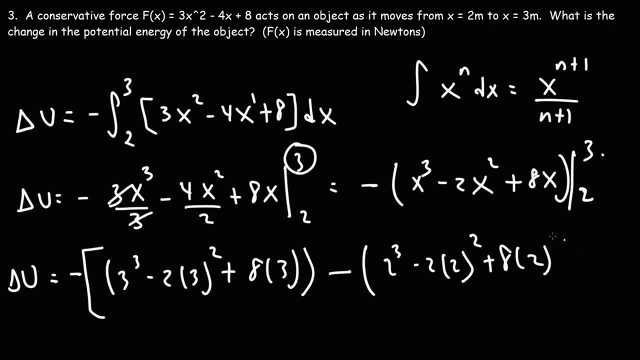 2 times 2, squared plus 8 times 2.. And don't forget about the negative that's on the outside. So 3 to the third power is 27.. 3 squared is 9 times 2.. That's 18.. 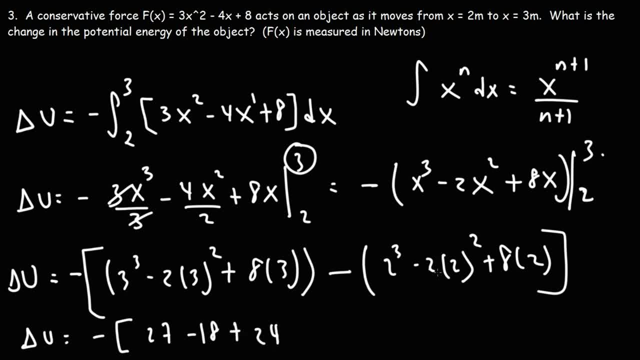 8 times 3 is 24.. Now, 2 squared times 2 is 8.. That's going to cancel with 2 to the third, So we're just left with negative times: 8 times 2, which is 16.. 27 minus 18 is 9.. 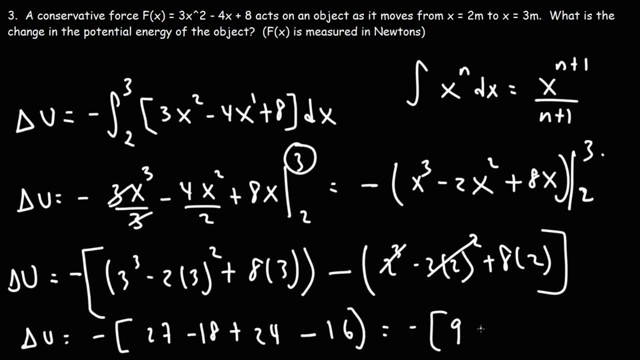 And 24 minus 16 is 8.. 9 plus 8 is 17 times negative. So we get negative 17 joules. If the force is in newtons and the displacement is in meters, the potential energy will be in joules. So that is the. 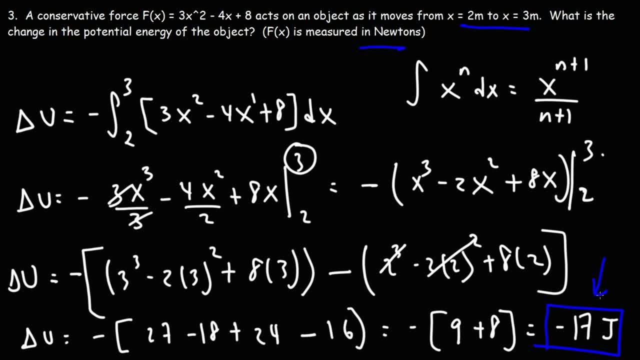 change in the potential energy of the object, It's negative. So as x increases. or if the displacement vector is to the right as we go from 2 to 3 and the potential energy change is negative, which means potential energy is decreasing, what can you say? 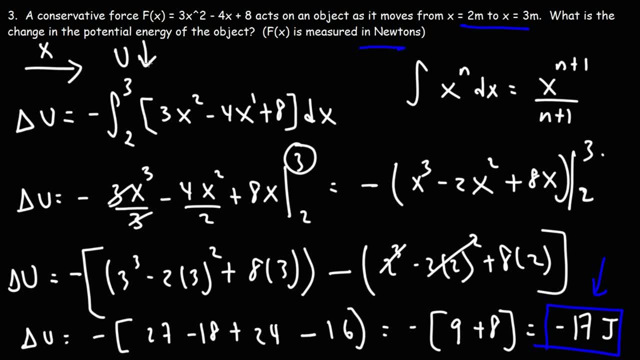 about the overall direction of the force in the x direction. Is it to the right for the most part, or to the left, Because the potential energy is decreasing as the displacement is to the right, the force is going to be in the same direction as the displacement vector. 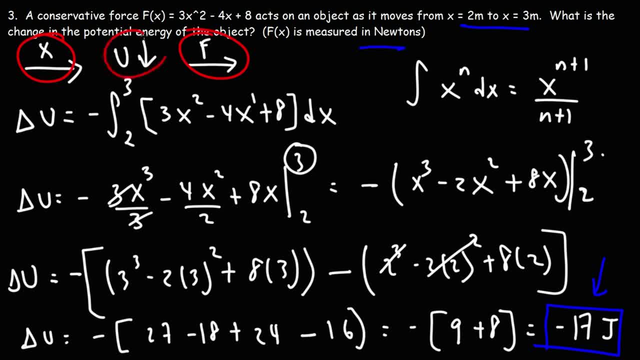 When these two are in the same direction, the potential energy decreases, And if we were to plug in 2 into f, we would get a positive number, And if we were to plug in 3, that would give us a positive number as well. So 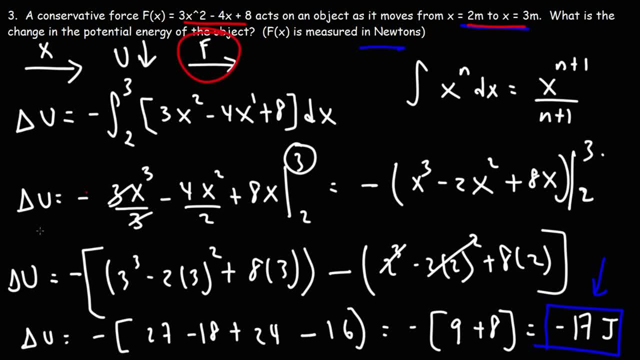 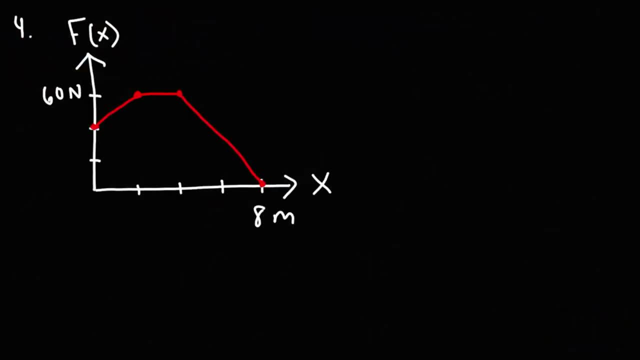 just by plugging these numbers into the function we'll get a positive value for f. But if you know the displacement vector and whether or not the potential energy is increasing or decreasing, you could determine the sign or the direction of the force vector In this example. 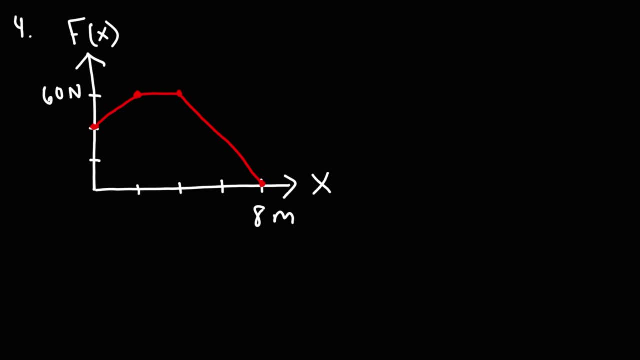 we have the graph of the force function as a function of x And we want to calculate the change in potential energy of this function as the object moves from a position of 0 to 8 meters. Feel free to pause the video Now we know. 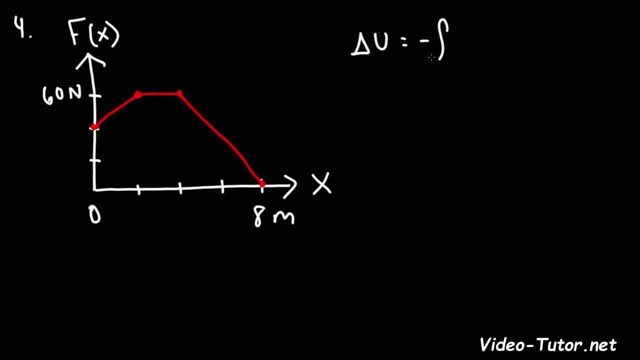 the change in potential energy is going to be negative times, the definite integral from a to b of the force function. Now this definite integral is also equal to the area under the curve. So for a force displacement function, or rather a force position function, the change in potential 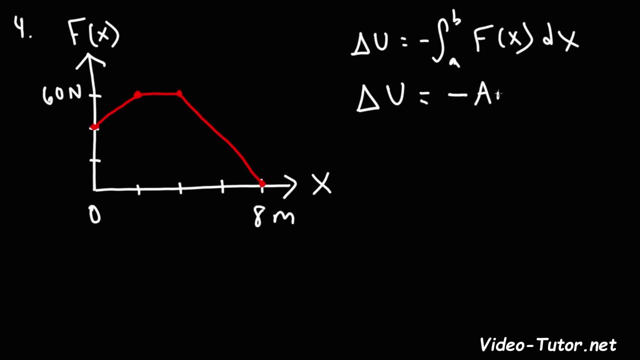 energy is going to be equal to negative times the area under the curve. So let's calculate the area under the curve. I'm going to break this up into rectangles and triangles. So this is 2,, 4,, 6, this is 20,. 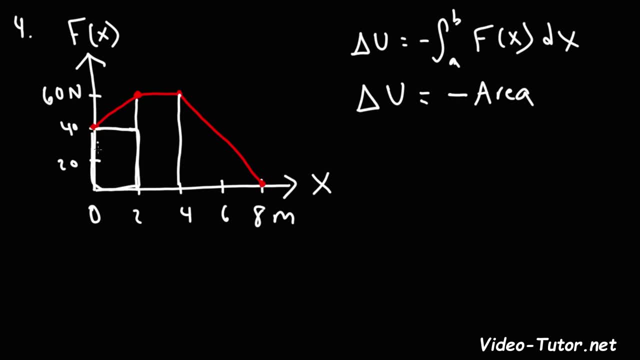 this is 40. So for this rectangle here we have a length of 2 and a height of 40.. 2 times 40 is 80. So that's going to be 80 joules. For the next rectangle, we have a length of 2.